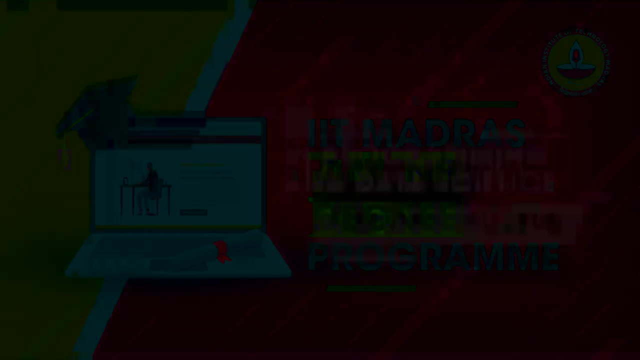 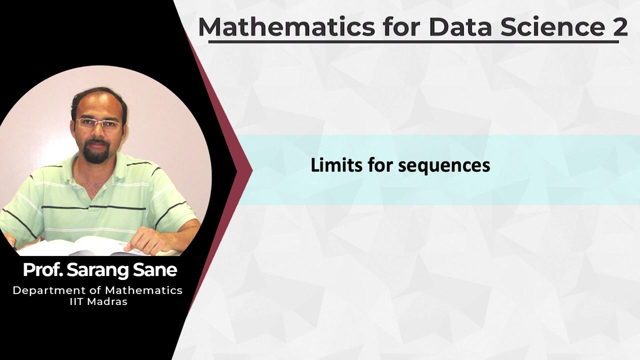 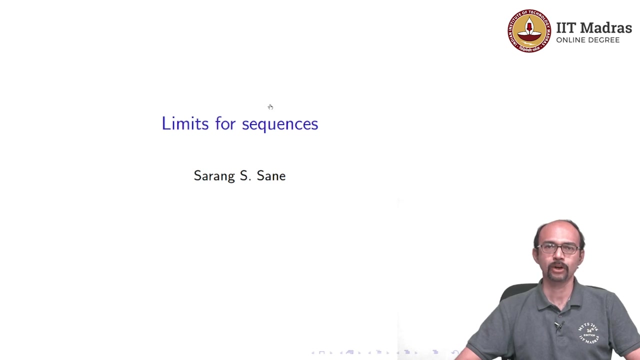 Hello and welcome to the Maths 2 component of the online BSc program on Data Science and Programming. In this video we are going to talk about limits for sequences. In our previous video we have seen the idea of tangents And we saw that it is a really tricky question. 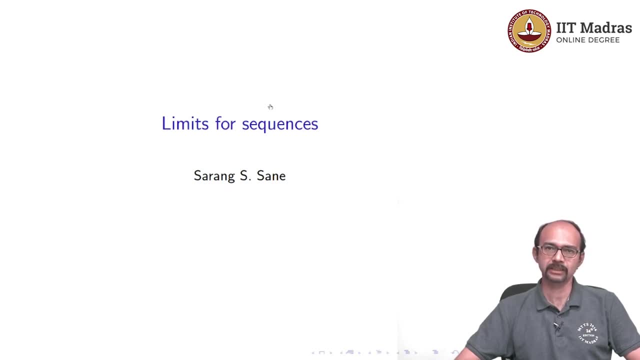 as to what is a tangent and when does it exist? And we saw some examples towards the end which motivated that there is some more depth to that question And indeed this is a deeper question than it seems just from geometry, And for this reason one has to start getting. 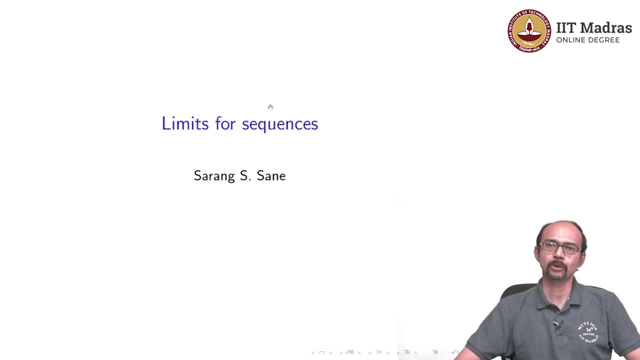 into what is called calculus. So we have seen calculus in some form, presumably in high school, or maybe you are not, But presumably you may not have seen what the form that we are going to use it in now. So we are going 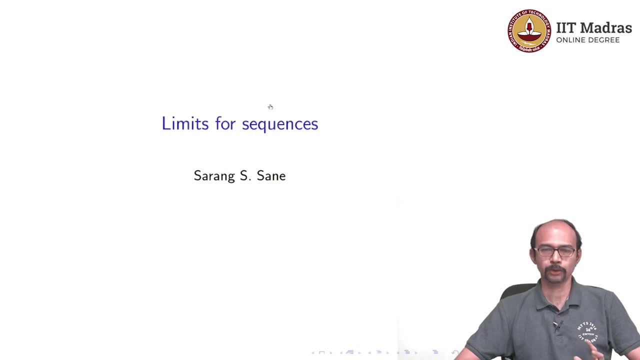 to do a little bit of. we are going to develop a little bit of theory, And we will then use that theory to get our handle on the idea of tangents much better. So the we are going to approach it from something called the notion of tangents. 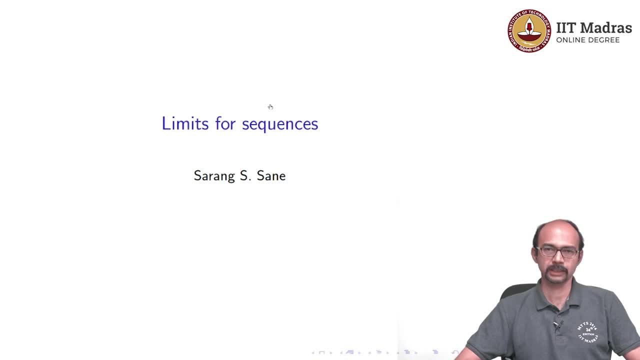 So let us start first with the notion of the definition of T tangents. Now, what I am going to do is: what is the definition of tangents, or crossing? I mentioned that star Lie. I am going to explain fast. So, as you can see, we are going to look at the 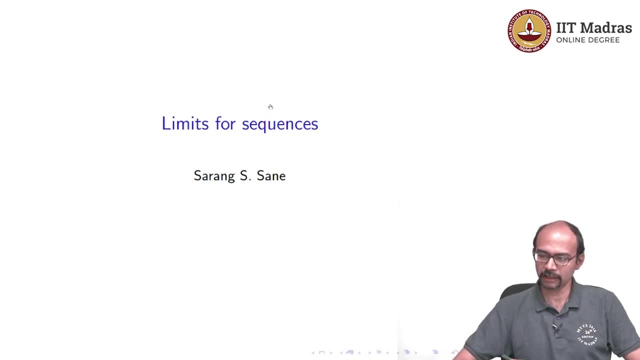 geography of the degree of T tangents, and it will be less and less realistic. So we will want to design ourSTICK plan for this type ofFORE Yong. so I am going to give you some one method of running » all the way to, basically, GoogleSkills2, where it will 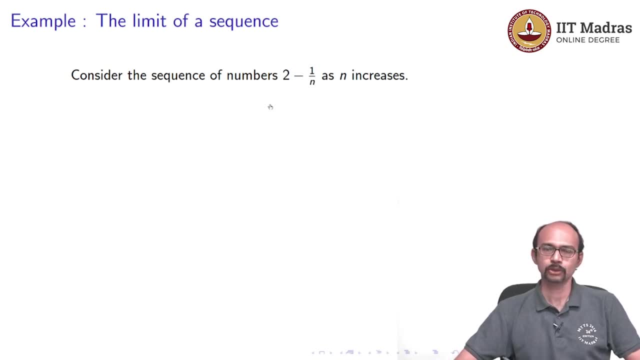 get a better search of all the values in a very intuitive way. Yes, it is a very gravy way of running it, So this new갑 실 videos will be quite interesting video and I will use some best Hiç Youth inputs calling » reg' english and the Julie Way to the hardwoods file. 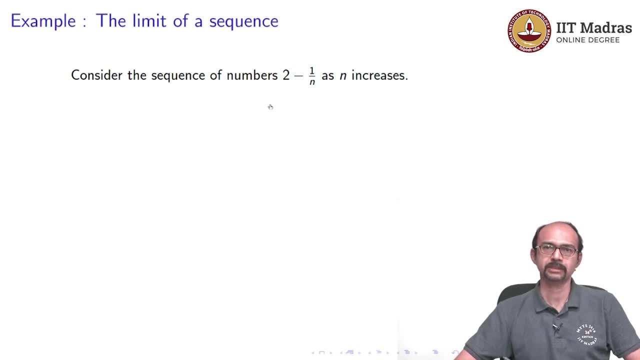 this. maybe I should first ask what is a sequence, or I should first mention what is a sequence. So a sequence is a set of its, an assignment. for each number n, there is some corresponding number which we will call maybe a n. So in this case, a n is 2 minus 1 by n. So as n increases your 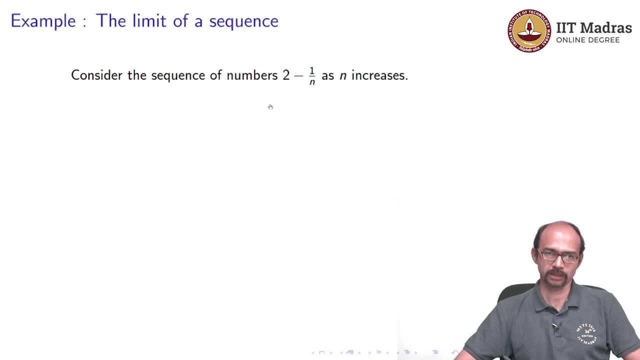 sequence of numbers. a, n also changes and the question is: as n increases, what happens to this sequence of numbers? So one possible sequence of numbers is: let us say, 1,, 2,, 3,, 4,, 5,, 6.. This 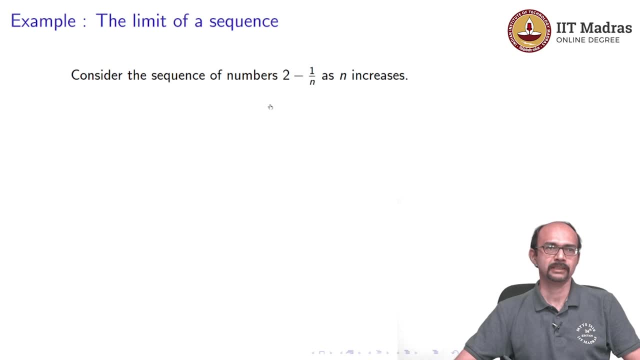 is a sequence of numbers. Another possible sequence of numbers is, let us say, 1 minus 1, 1 minus 1, 1 minus 1. that goes on. So you could write this in a more tangible fashion as: minus 1 to the power n. 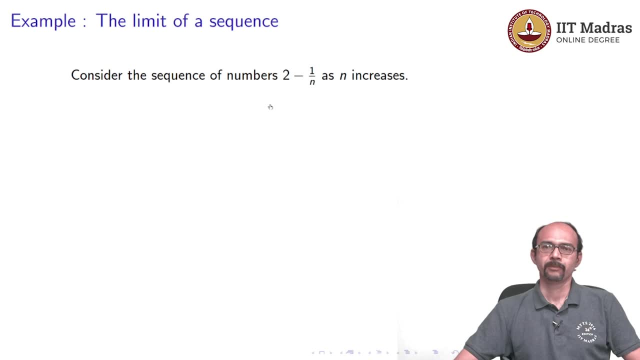 Or another possible sequence of numbers is, let us say, half one-fourth, one-eighth, one-sixteenth, one by 32,, one by 64. If you know these numbers well, you will- you can tell that this is the sequence 1 over 2 to the power n. 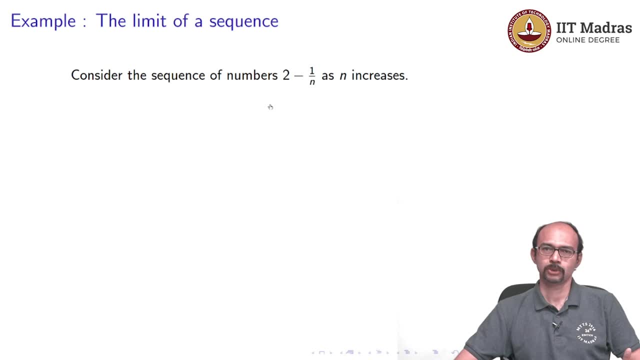 But of course the sequence need not have a closed form, So the sequence could just be for: for each n you associate some number. that is it. So that is the sequence. So here is the sequence: 2 minus 1 by n. And let us ask what happens as n increases. 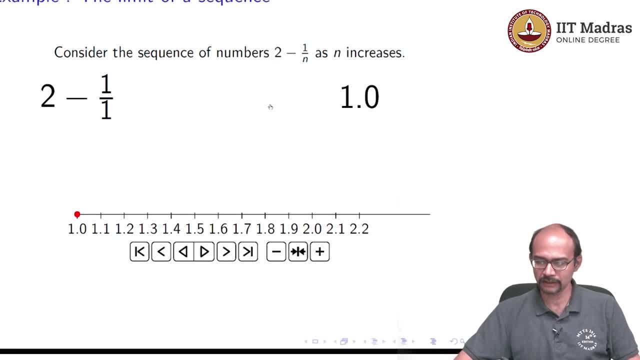 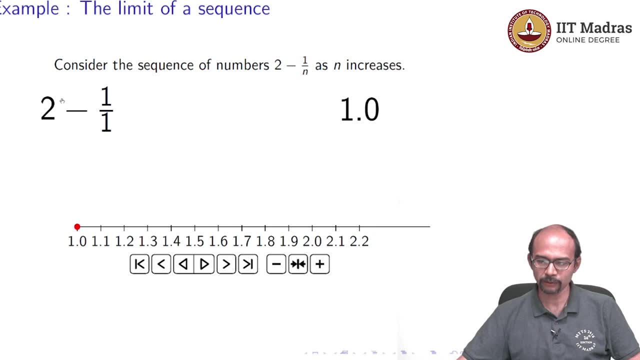 So if you look at what happens as n increases- let us try to play this video and see what happens So as n increases- you can see on the left hand side you have 2 minus 1 over n. So you can see what is n. as n increases it will change. For example, the next term is 2 minus 1 by 2.. 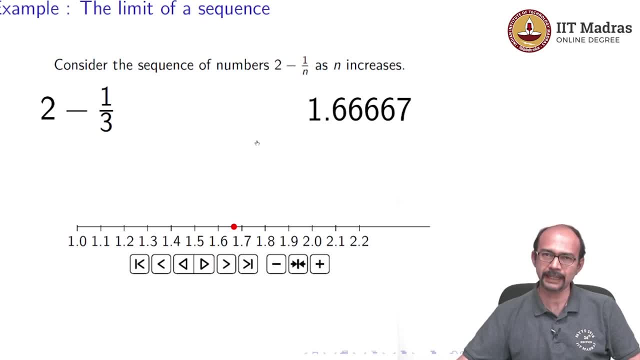 the term after that is 2 minus 1 by 3, and its value is on the right hand side. So keep track of what happens to the value as your n changes. Now let me play this So as you can see, as your n is increasing. well, you have 1.98,, 1.988,, 1.989,, 1.99,, 1.993,. 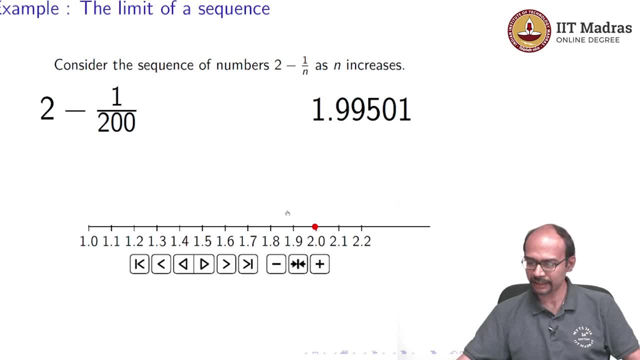 1.994.. So you can see this is increasing. and here below is the real line, the part between, let us say, 1 and 2.2, and if I play that again you can see how the geometry of the sequence. 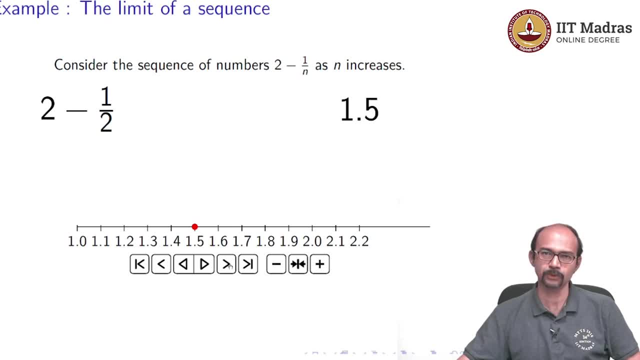 So the first term is 2 minus half, which is 1.5.. The next term is 2 minus one third, so that is 1.66.. And if I play it further, you can see that the red dot comes closer and closer. 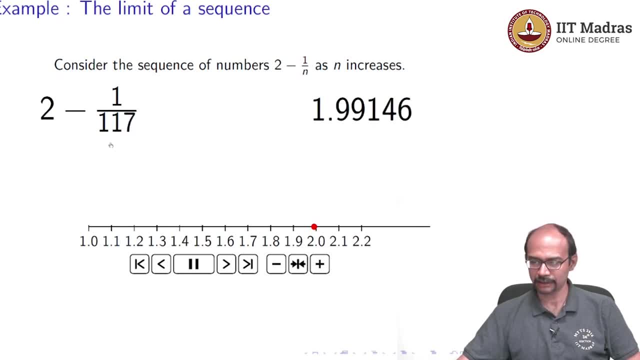 and closer and closer to 2, and as your n increases- now it is 130,- it is going to be pulled to turn to 0.. It is going to be pulled to 2.5, and now it is going to be pulled to 1.6. 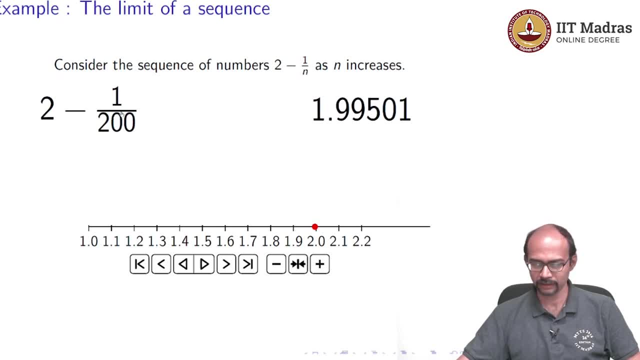 to come very, very, very close, as it is 200, where I have stopped the sequence, it is really close to 2, it is 1.995.. So you can tell that, as n is going to become very, very, very large, this sequence is going to come very, very, very close to the number 2.. 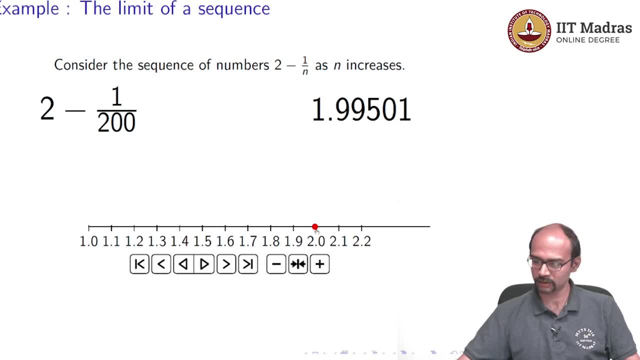 So, in other words, this red dot is going to come even closer to this point 2.. That is what this means geometrically, and that is what it means in terms of your algebra or your numbers: that it is going to come close to the value 2.. 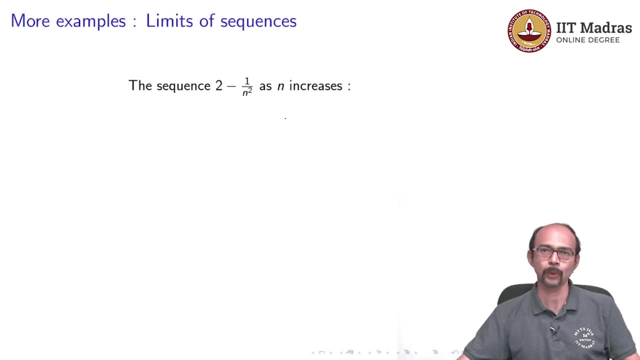 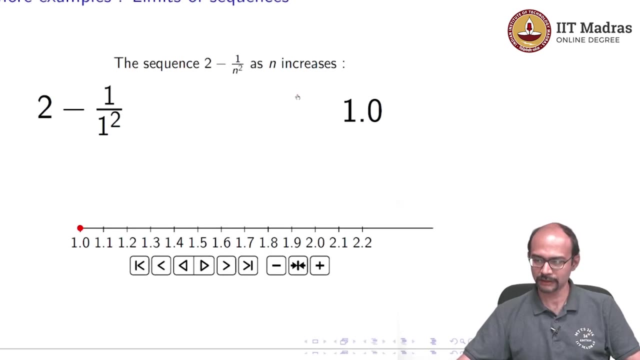 So let us do the same thing for the sequence 2 minus 1 by n, squared. I want to do this because I want to see the speed with which this works. So if you do it for 2 minus 1 by n, squared. 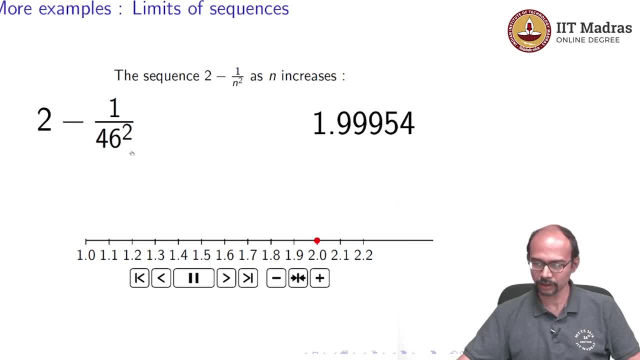 well, you can see, it went very, very, very fast. So it is already at 50 and we are at 1.9996.. Let me replay that. So here is your first: 1 minus 1 by 1 square, so the number is 1 and the 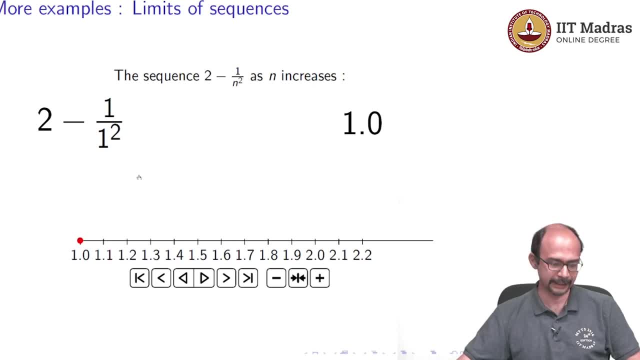 red dot is at the position 1 on the real line And as you go ahead you get 2 minus 1 by 2 squared. That is 2 minus 1. fourth, 2 minus 1 by 3 squared, 2 minus 1. ninth, and, as you can see, 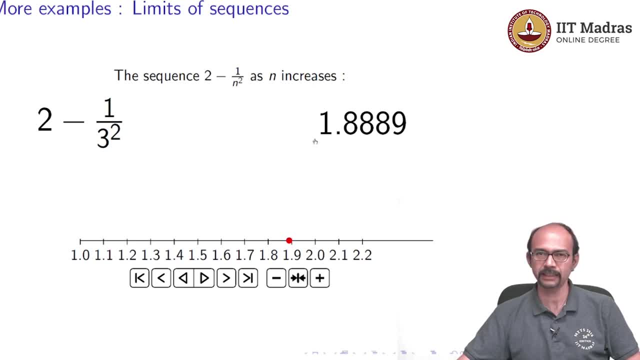 it is already on. the third term itself is 1.8889.. It took much longer, for the sequence is 1 by n and another few terms and it is 1.97.. So it is very close And if I play that, 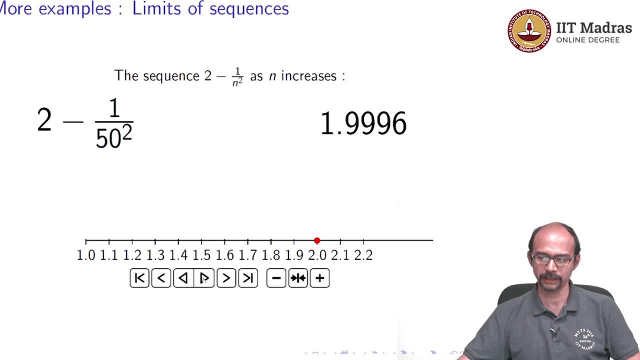 29,, 30 and look at what is happening: it is 1.999 already. So this number, as you can see it comes very close to 2.. In fact, if you look at the line, our points are not fine enough to. 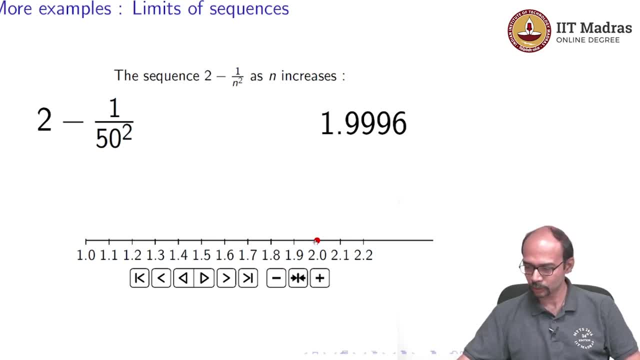 distinguish between these numbers 2 and 1.9996.. So this red dot is already, it seems, as if it is sitting at 2, but it is not. It is actually very close, but not exactly 2. And you can see as n. 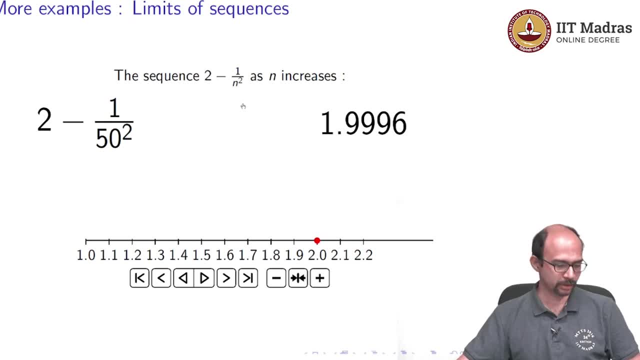 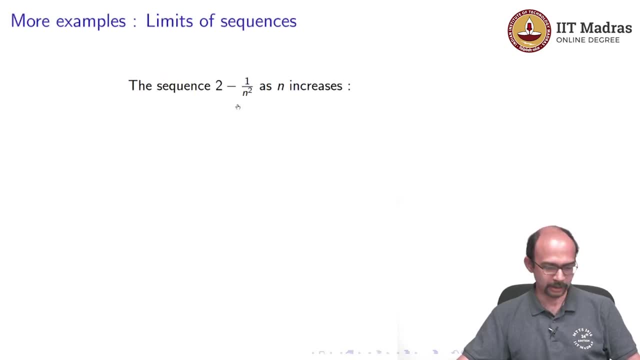 increases. this sequence is going to. this sequence of numbers is going to come closer and closer and closer to the number 2.. Let us do one more example just to motivate further what is happening. So here is a slightly more complicated sequence. It is a sequence 2 minus. 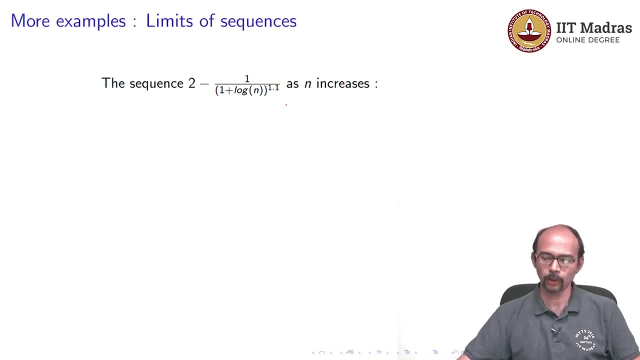 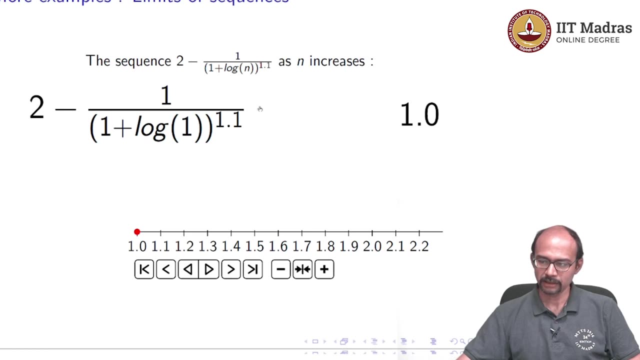 1 divided by 1, plus log n to the power 1.1.. And to check what is happening. well, we again have the same counter, And this time I am going to play it. going to play it for a much longer time. 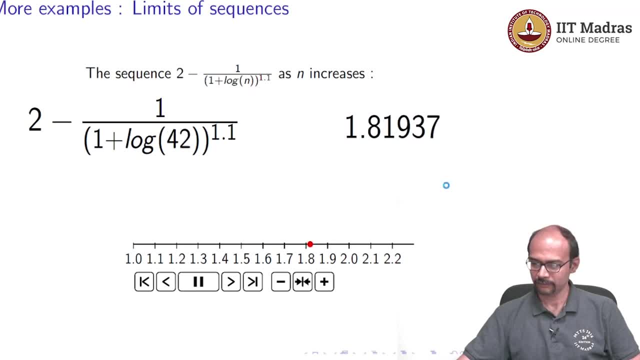 and you will see why. Now it is 1.83,, 1.84,. look at that red dot. it is moving very slowly. It is moving, moving, moving. but now it is very, very slow And we are already well past where we were in our previous sequences. 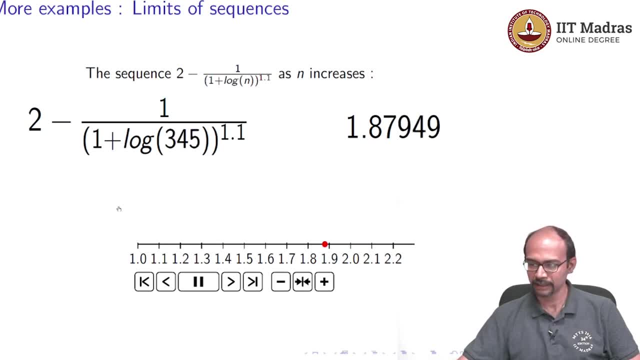 We are now at closing on 300, still not past 1.9.. In fact, at this point, if I stop it, it is at 367,. you may feel well, maybe it is not going to 2,, maybe it is. 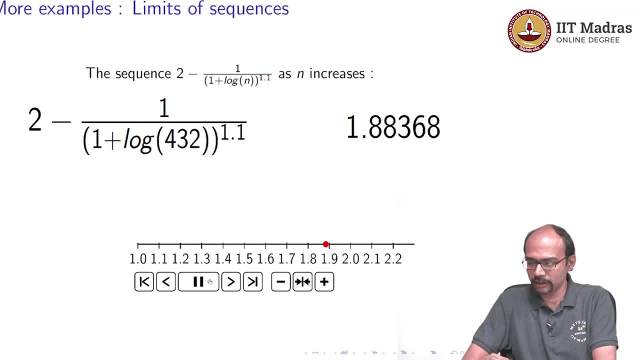 going to stop before 2.. So well, let us play it further. And now it is coming closer to 1.9,, it is 1.88.. But those numbers are moving very slowly. It has passed 500 already. 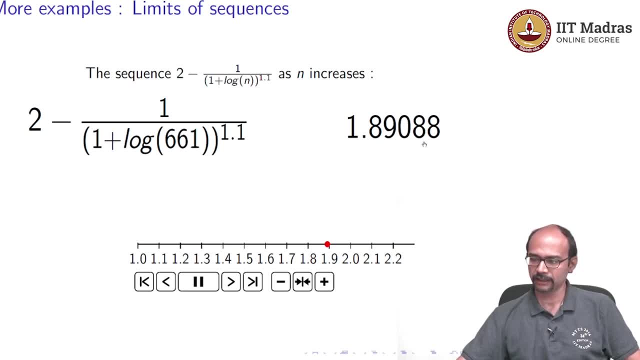 And that red dot is closing on 1.9.. So I want you to have a visual feel of what convergence of sequences limits of sequences. So here we are now where we are at 9, N is 800 or 900 and we are still not past 1.9., But you can see it is coming close. 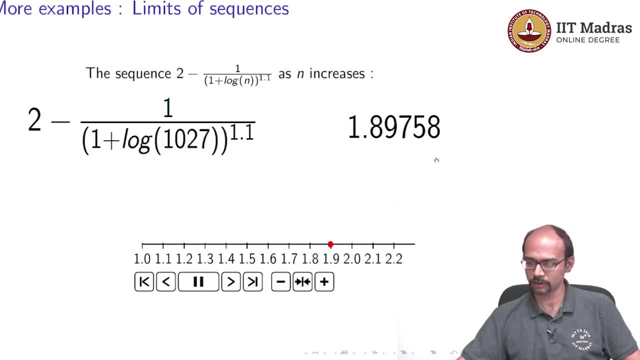 Now we are going to come closer and closer and closer, And you probably feel that very soon, we will cross 1.9. Indeed, we are very close to doing that. There we are, we have crossed 1.9. And now the red dot is on the other side And very, very, very slowly. 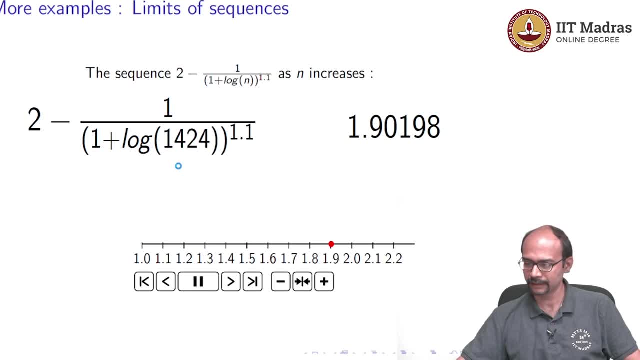 you can see n is very large. now it is close, almost 1400.. It is moving, but now it is very slow still at 1.90.. And we can keep going. I will just take you till the end. 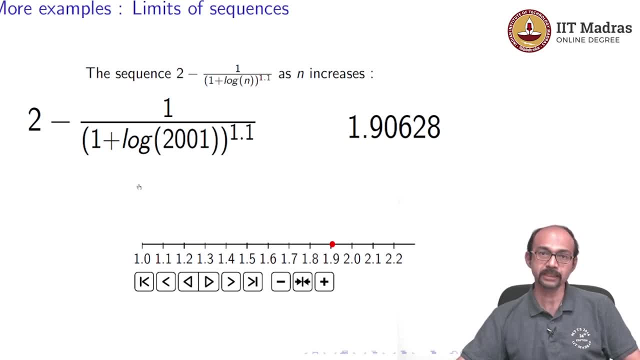 And I have stopped at 2000,. meaning, when I say I have stopped at, or rather 2001,, I have stopped at the 2001th element of this term, of this sequence, or element in this sequence. So what is that? 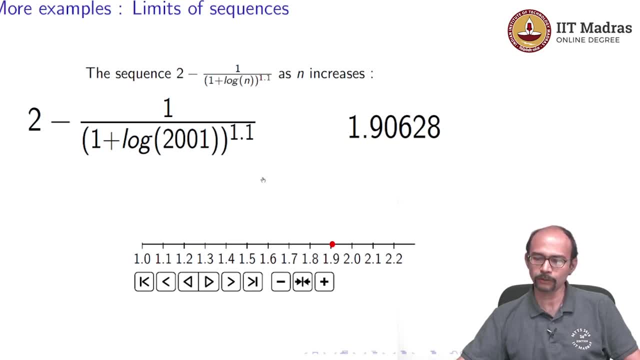 term. It is 2 minus 1 by 1 plus log of 2001,. the whole to the power 1.1, rather strange looking. And where have we gone? We have come till 1.90628.. So this is a very slow moving sequence. 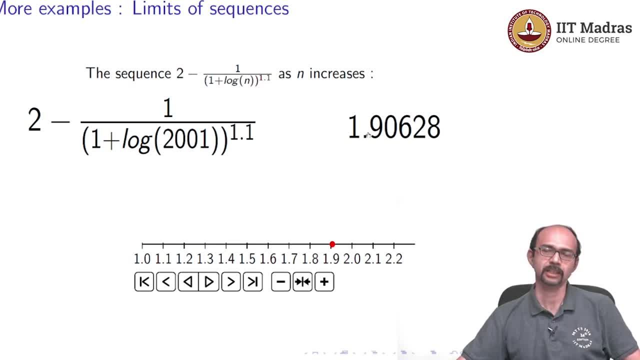 But my claim is- and I will encourage you to check that this sequence: indeed, as your n becomes very, very, very large, this number will come very, very, very close to 2.. So this number is going to come very, very, very close to 2, or in other, 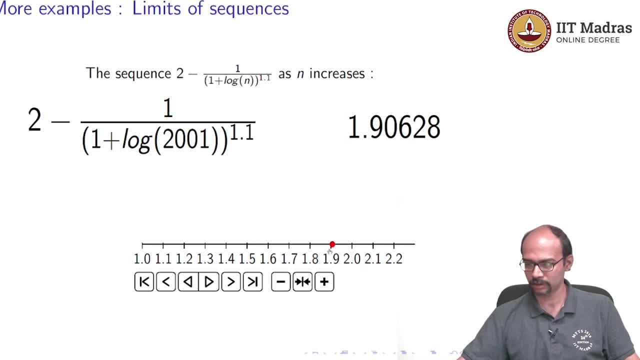 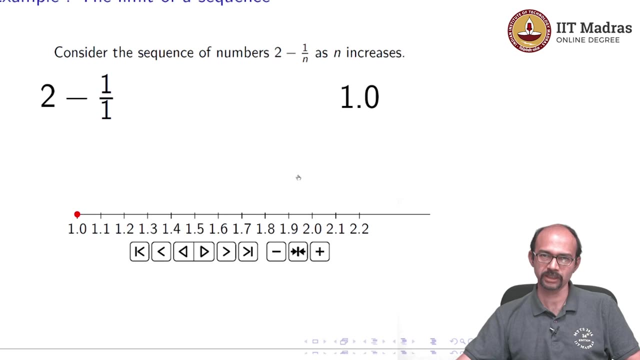 words, this red dot, this red point, which denotes that sequence is going to come very, very, very close to the number 2.. It will keep moving, but it is going to come very slowly. So first sequence 2 minus 1 by n that we had. this was a reasonably fast moving sequence. 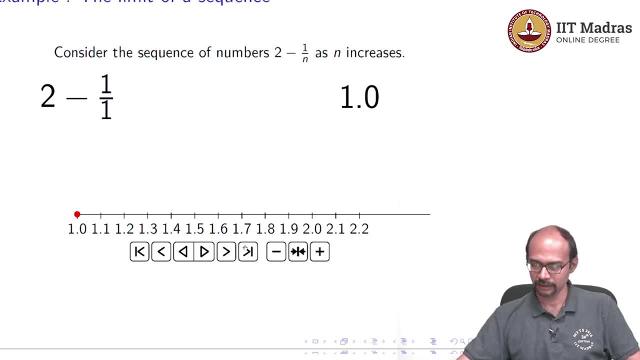 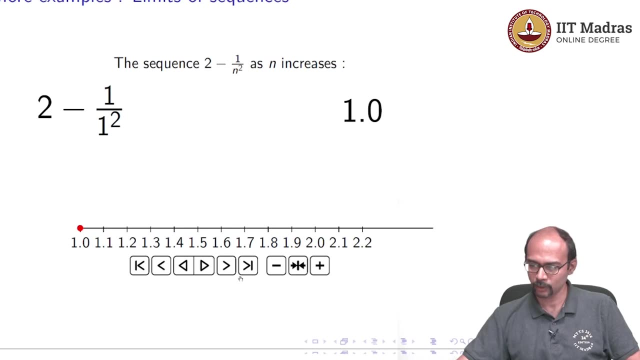 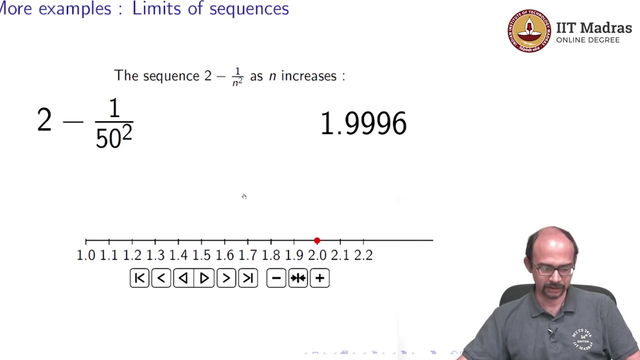 Within 200 terms, we came to 1.995.. The second sequence: it was 2 minus 1 by n squared, Within 50 terms, we came till 1.996.. And the third sequence: well, we went till the 2001th term. 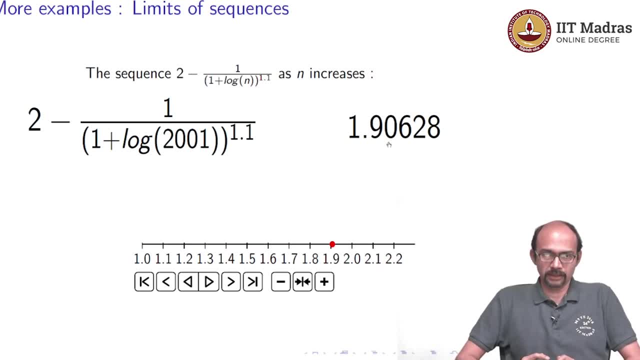 and we still had 1.906.. So this is. there is also an issue of how fast does it? does a limit, does it approach a limit? And the first one is reasonable, the second one is fairly fast and the third one is relatively slower. So you may see these ideas coming up. 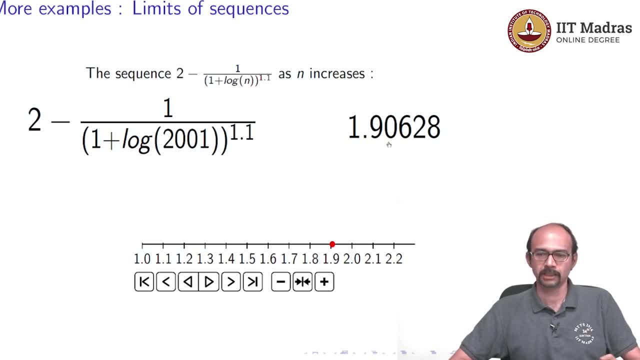 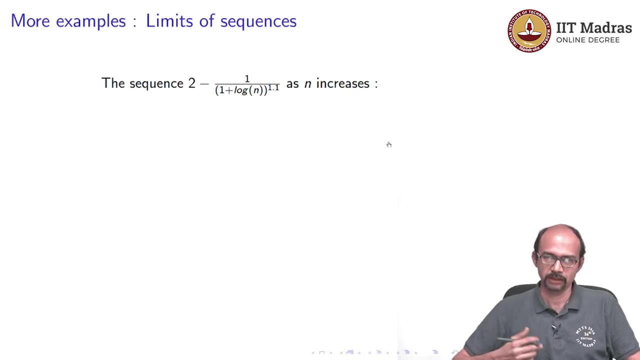 again in some other course, completely unrelated to what we are doing now. And, in case you do, do that in the programming part maybe. And in case you do, you may want to think of this again. So, with that motivation, for what is the limit of a sequence, let us define this. 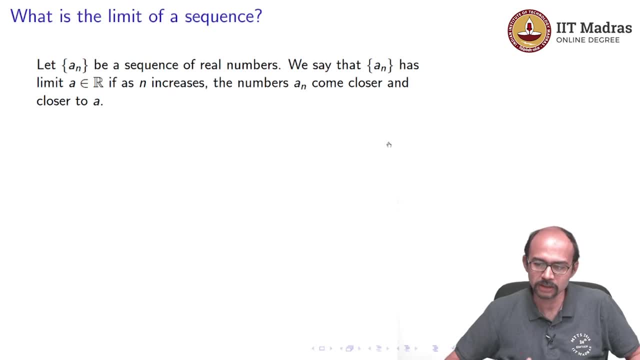 explicitly. So what is the limit of a sequence? So let a n be a sequence of real numbers. We say that a n has limit a, which is some other real number, or it could be one of the real numbers already appearing in your sequence. If, as n increases, the numbers, a n come closer. 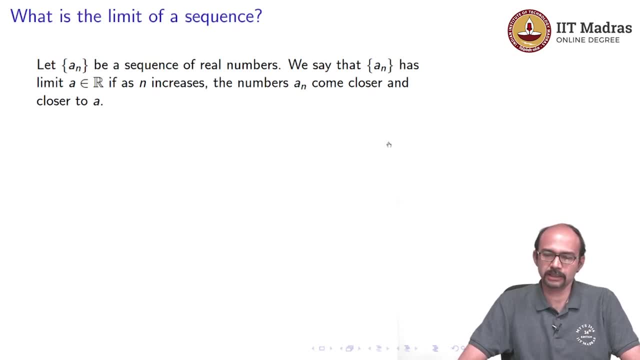 and closer to a. So that is the intuitive definition of the limit of a sequence. Now it is natural to ask: what do we mean by closer and closer? and that is something I am not going to get into. There is a more formal, abstract definition, mathematical definition, 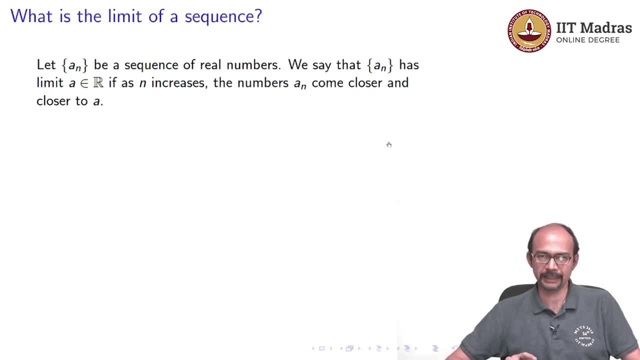 for what it means to come closer and closer, and I am not going to get there. So we are going to just see, enough to be able to make out what is going on. We would not be doing details here. What is? what are other ways of saying the same things? So 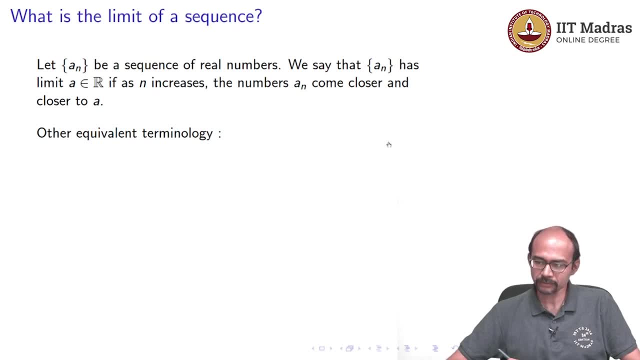 this. so the above statement was that the sequence has limit a. if this happens, What is other equivalent terminology? a? n tends to a. that means the same thing: that the sequence a? n has limit a. So what is the other equivalent terminology? a? n tends to a. that means the same thing. 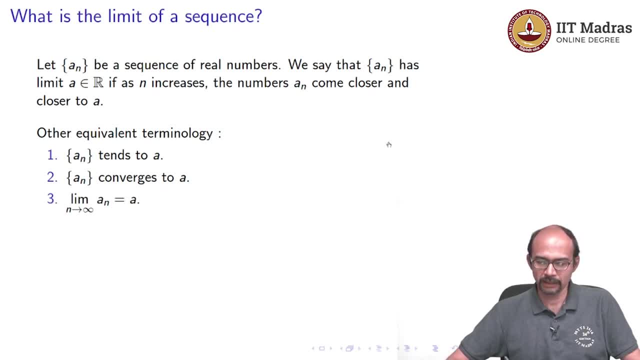 a n converges to a again same thing. Limit a n is equal to a. that is notation you may come across if you read books or if you happen to look on the internet. a n again, arrow a again means that the sequence a- n has limit. a a n, arrow a and above that n tends to infinity. 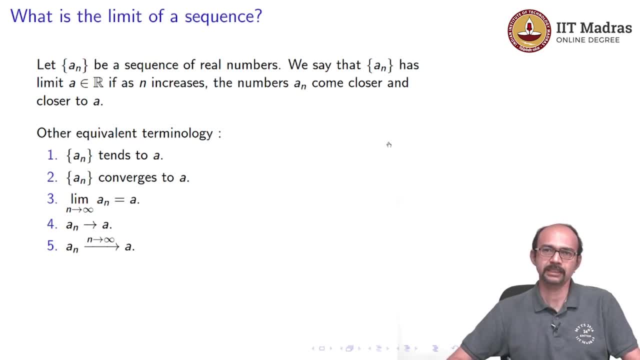 or sometimes it is below that. So that again has the same meaning that the sequence a has a, n, has limit a or just simply limit a n is a. that also means that the sequence as n tends to infinity. the sequence has limit a, or sometimes you may have the same thing with the bracket or with the n. 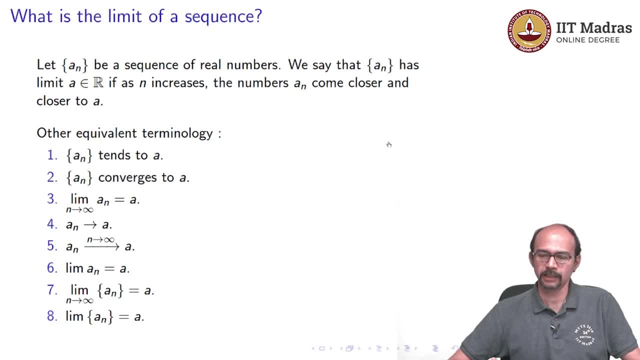 tends to infinity or without the n tends to infinity. So all of these are notations for the same statement. So all of these mean the same thing. So all of these mean that the sequence a- n has limit a. So I may often use the first two: a? n tends to a or a? n converges. 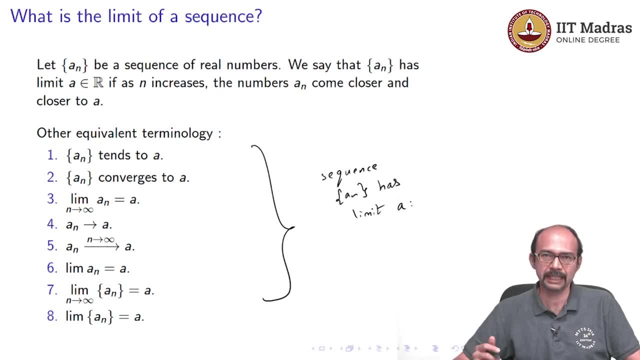 to a in place of a. n has limit a, And do not be confused by that. that is exactly why I had this slide up. So what does this mean? Let us come back to that, which is the one, which is the more important part. It means that as n becomes larger and larger, these 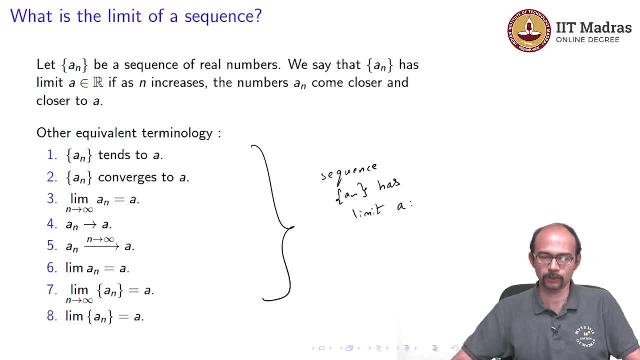 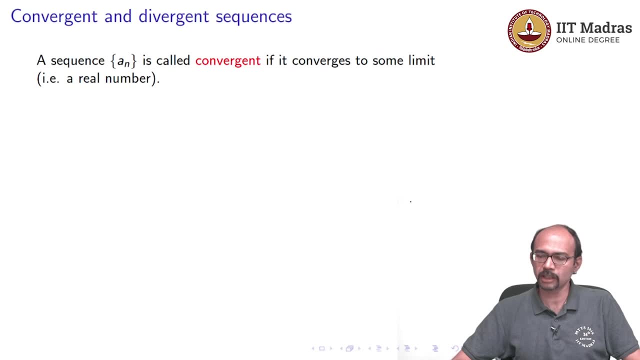 numbers a- n come closer and closer to a. That is what you have to take home from here. Let us do some more terminology. A sequence a- n is called convergent if it converges to some limit. So by limit we mean some real number. So for example the sequence 1 by 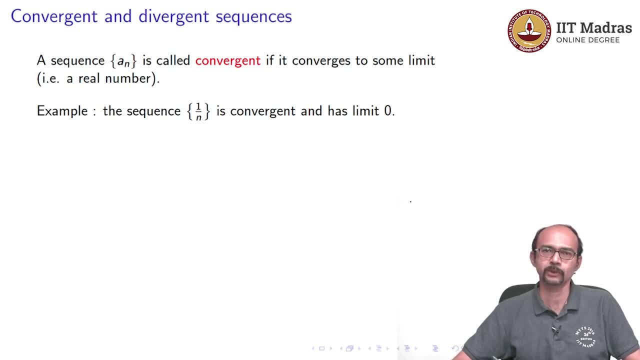 n is convergent and it has limit 0. If you look at the sequence 1 by n, you will see. you can see that as n increases, n becomes very, very, very large. the numbers 1 by n become very, very, very small. When I say small, I mean they are positive and are small. 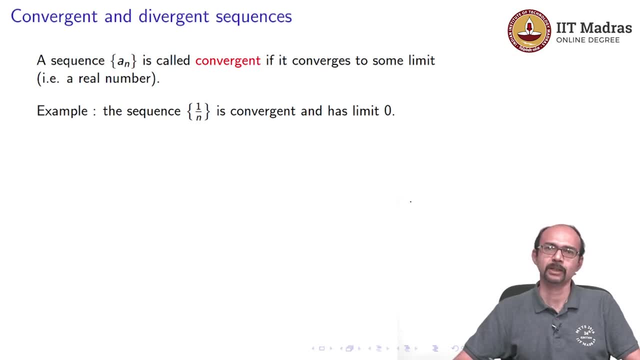 So as n becomes very large, the numbers 1 by n are going to come closer and closer to 0. So this is an example of a convergent sequence. A sequence- a, n- is called divergent if it is not convergent. If it is not convergent, it is divergent. That means these numbers. 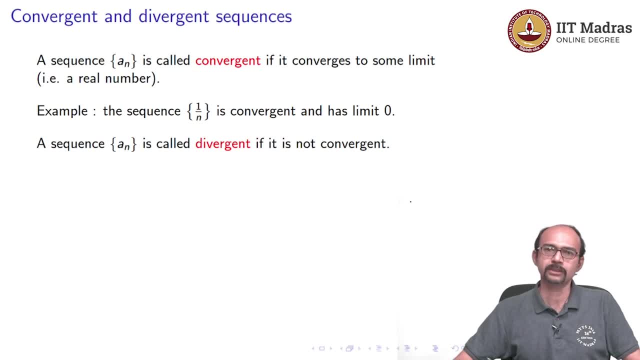 these numbers do not converge to a limit which is a real number, or do not converge at all. They may float around. So here is an example. This is an example that we saw right at the beginning of this video. The sequence 1 minus 1 to the power n is divergent. What is the 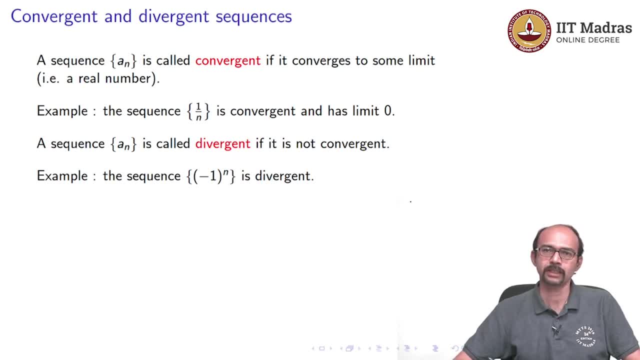 sequence. Well, the first term is minus 1 to the power 1,, that is minus 1.. The second term is minus 1 to the power 2,, which is 1.. Third term is minus 1 to the power 3,, which. 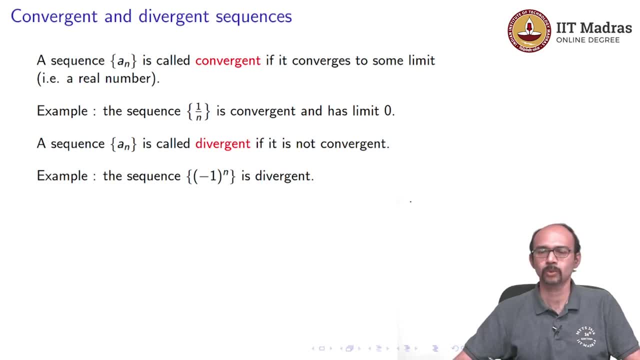 is minus 1.. So this sequence is: minus 1, 1, minus 1, 1,, minus 1, 1.. So this sequence is what is called oscillating: It oscillates minus 1, 1,, minus 1, 1.. So clearly this sequence does. 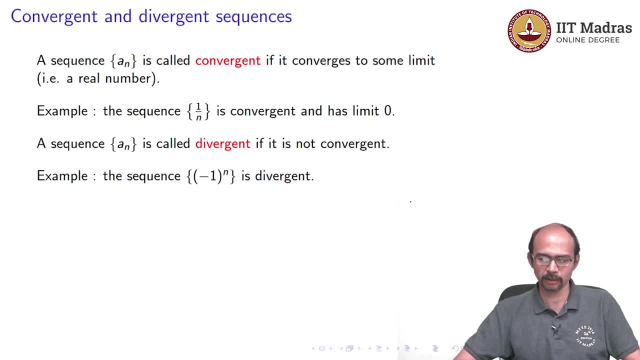 not have any limit. It is not coming close to any real number. So this is an example of a divergent sequence. We will come to more examples, But let me define what is called a subsequence of a sequence. So a subsequence of a sequence is a new sequence formed by possibly excluding some entries. 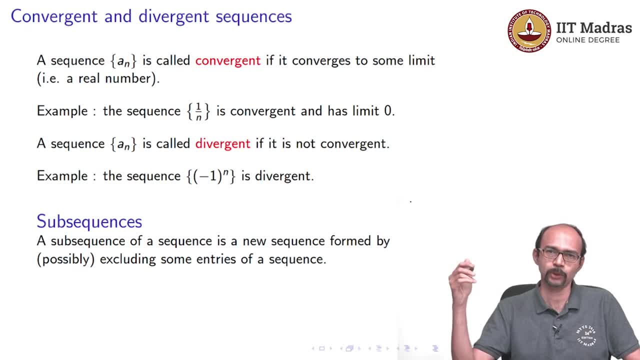 of a sequence. So if you have a sequence, so you have A1, A2, A3, A4, you have this sequence of real numbers and you drop some of those. You just take, let us say, A1, A4,. 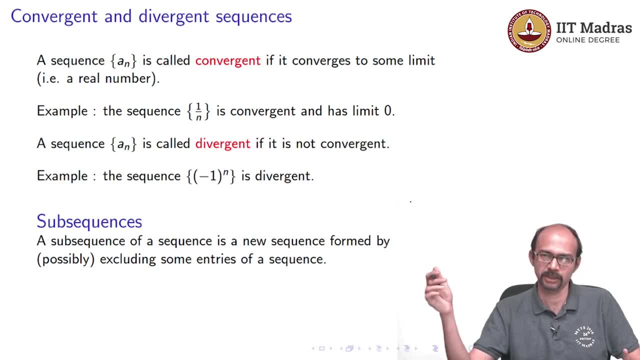 A20, 800, A1 million and so on in some prescribed order. So whatever you get is a subsequence of the sequence. So some A1, A2, A3, A4, A4, A2, A1 million. Here you have some real numbers. 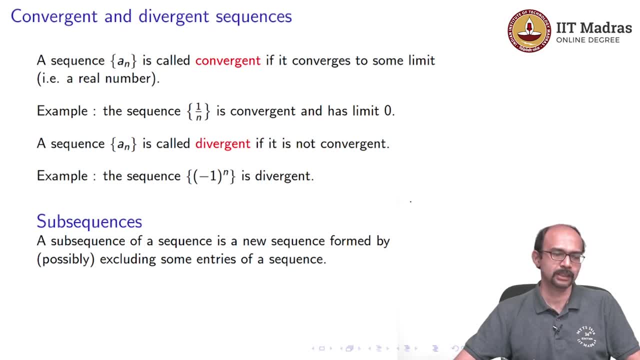 So some often what you do is you drop some interesting terms which are given by some mathematical way. For example, you can say: let us take all the odd part of the sequence, so that means you take the first term, third term, fifth term, seventh term and so on. or you can say: take 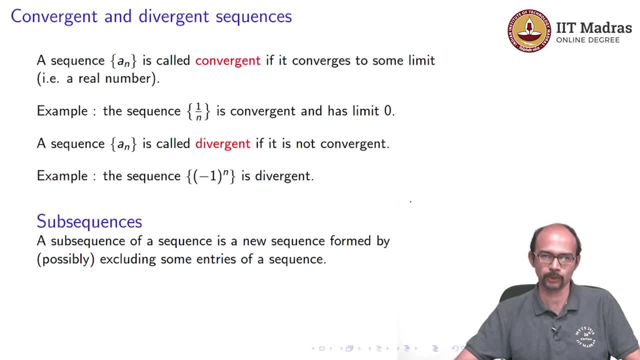 the even part of the sequence which is the second, fourth, sixth, eighth and so on. So here is an example. So here is your sequence: minus 1, 1,, minus 1, 1,. this is exactly the divergent sequence. 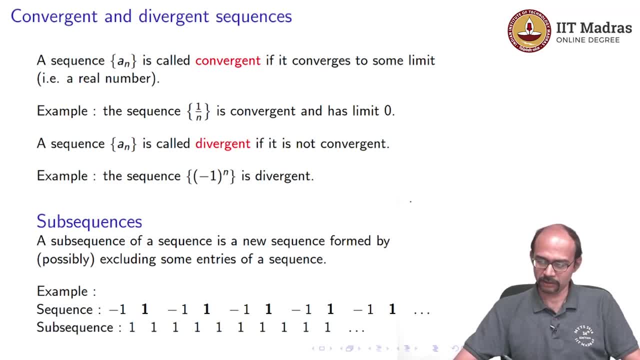 that we had above, and here is your subsequence, which is the one which is highlighted in that sequence. that is the even terms. so that is the second, fourth, sixth, eighth and so on, and if you do that, you get minus 1 to the power 2, minus 1 to the power 4, minus 1 to 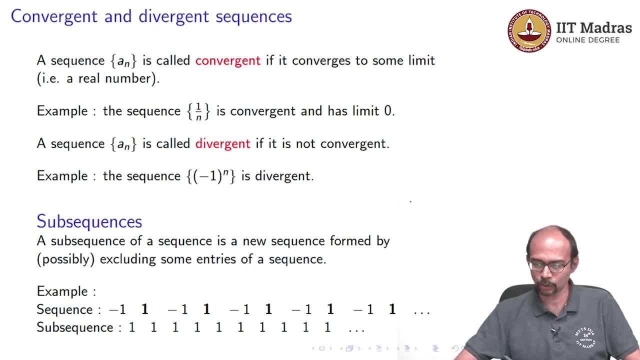 the power 6 and so on. So those give you exactly ones. So your subsequence is 1, 1, 1, 1, 1, 1, 1.. I could, of course, take other kinds of subsequence. 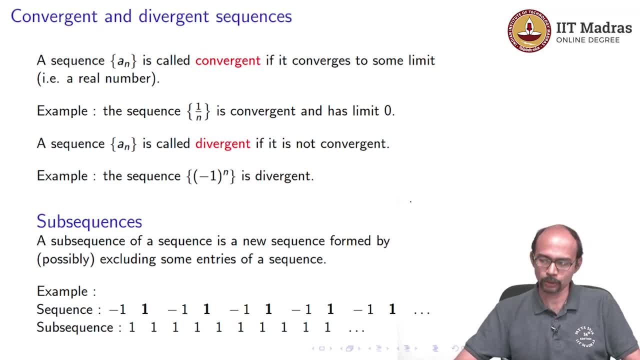 Subsequences which also have the same form. So I can take the, let us say, the fourth term, the eighth term, the twelfth term and so on. So minus 1 to the power 4n. So if you do that you still get the same numbers in your subsequence, but it is a different. 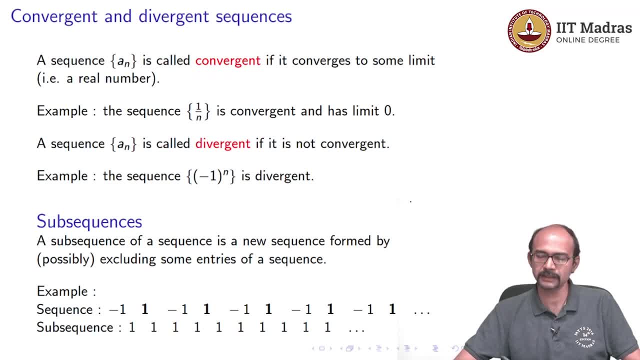 subsequence than the one written down, because, that is, this subsequence is the one obtained by taking the second, fourth, sixth, eighth and so on, whereas the one I just said right now is the one obtained by taking the second, fourth, sixth, eighth and so on. 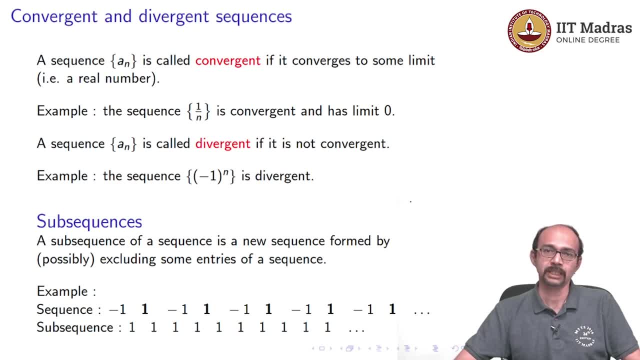 So as sequences, these are the same, but as subsequences of this sequence they are different. So some small quibbling here, and may not be important as we go ahead, but something to keep in mind as for those of you who are more mathematically inclined. 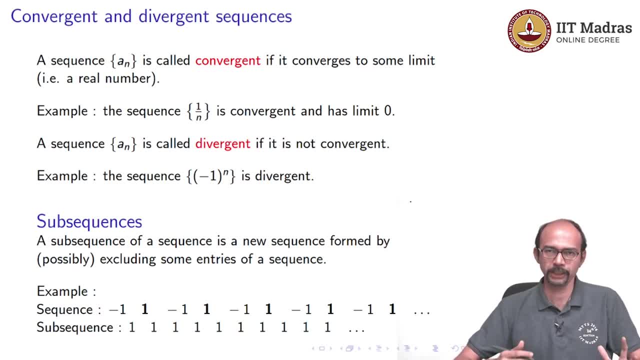 So I hope you have a feeling for what is a sequence, what is the limit of a sequence? when is a sequence convergent, which is exactly saying it has a limit? when is a sequence divergent, which means it does not have a limit? 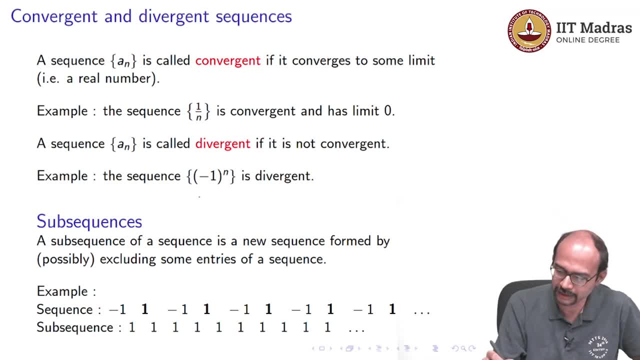 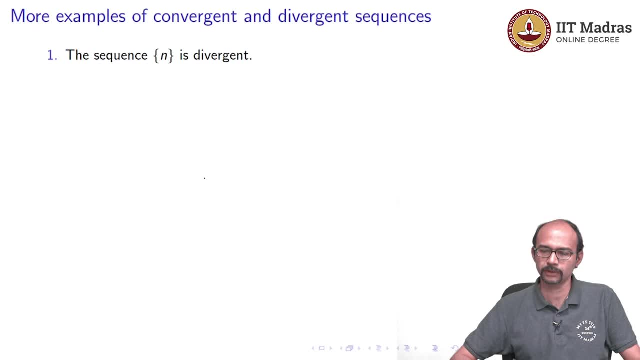 So we had this oscillating sequence. let us write down another example of a sequence which is- or maybe- I think next slide we have more examples. So here is an example of a sequence which is divergent, but in a different way than the previous one. 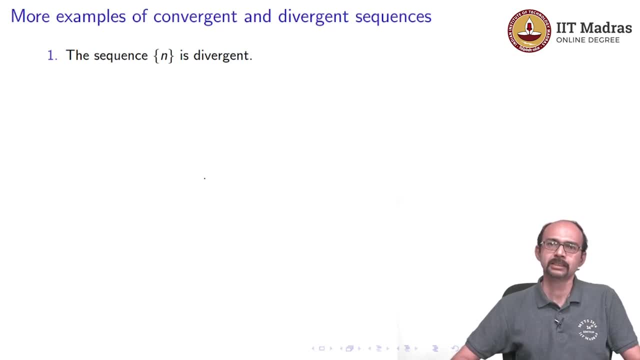 So the sequence n is divergent. What happens to this sequence n? So that is a sequence 1,, 2,, 3,, 4,, 5,, 6,, 7,, 8,, 9,, 10,, 11,, 12,, 13,, 14,, 15,, 16,, 17,, 18,, 19,, 20,, 21,. 21,, 22,, 23,, 24,, 25,, 26,, 27,, 28,, 29,, 30,, 31,, 32,, 33,, 34,, 35,, 36,, 37,, 38,, 39,, 40,, 41,, 42,, 43,. 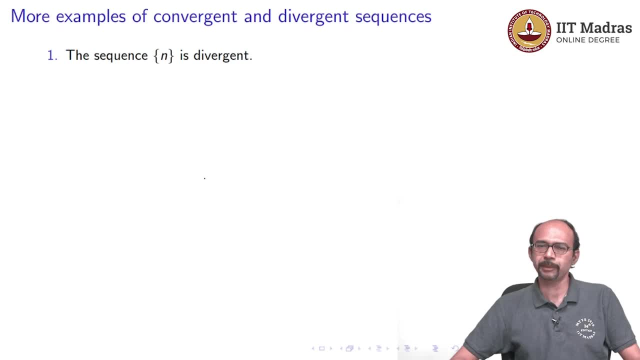 44,, 45,, 46. So this sequence does not have any limit. If you take any real number- let us say I take the real number 2 million- At some stage this sequence will go beyond this real number and it will keep going much. 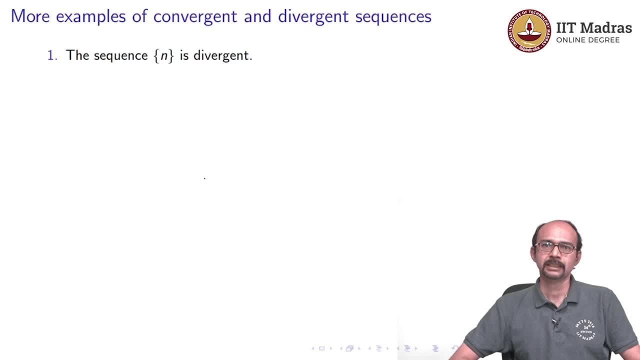 much, much beyond. It does not come close as n increases, So there is no real number to which it comes close. Now, some of you may of course have heard of this concept of infinity. In fact I have heard of it. I mentioned that concept previously, also in the slide where I defined terminology. 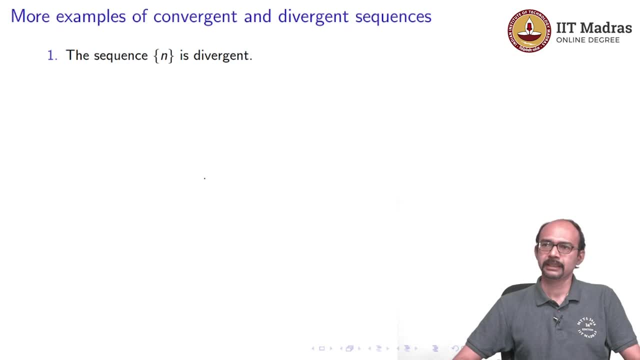 So infinity we think of as something which is very, very something larger than any number that we know, any real number that we know. So you can say that this sequence converges to infinity. So in this case, we can actually say that this sequence converges to infinity. 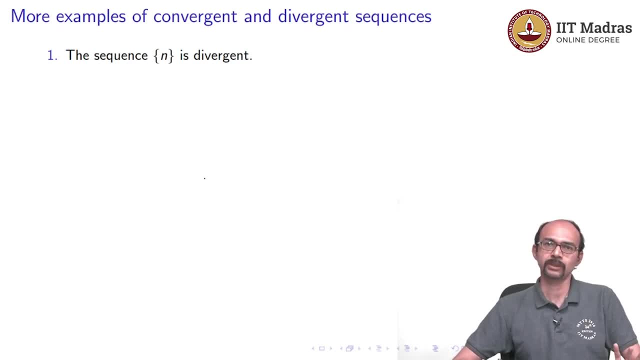 But as far as our notations are concerned, it is still a divergent sequence. So you could say it converges to infinity, you could say it diverges to infinity, or you could just say this sequence is divergent, which is correct. 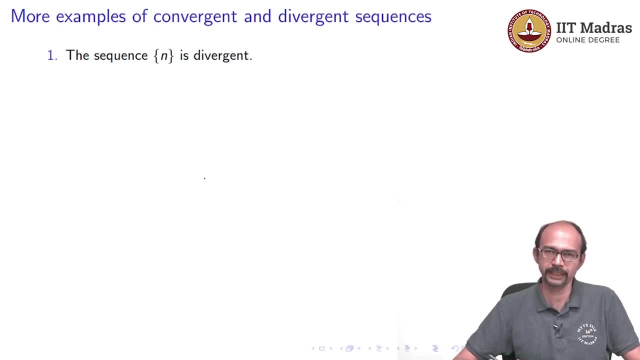 So the previous two things- saying it converges to infinity or diverges to infinity- say more than just saying it is divergent. But this sequence is divergent. So that is what you have to keep in mind: that it is divergent. 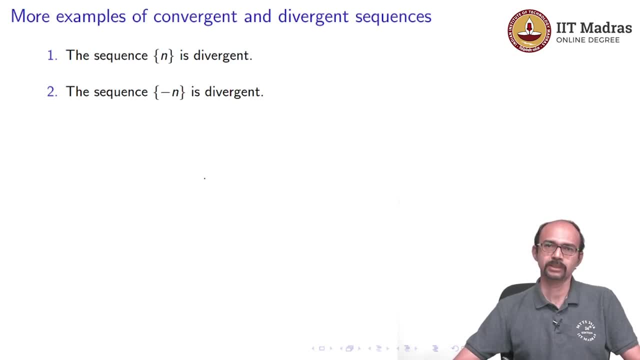 Same thing for minus n. The sequence minus n. Now, what is the sequence? What is the sequence? It is minus 1, minus 2,, minus 3,, minus 4,, minus 5,, minus 6,, minus 7, and so on. 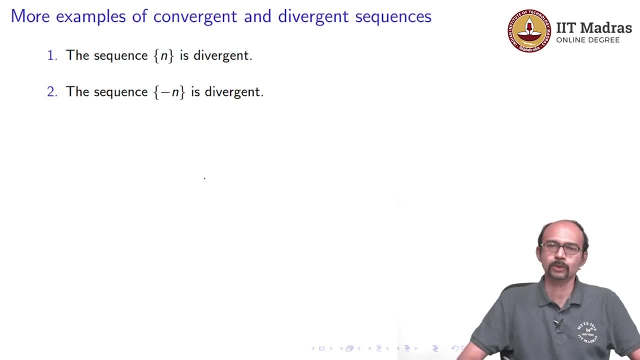 So, as you go ahead, this sequence is going to become, the numbers in the sequence are going to become very, very, very small. And when I mean small, I do not mean positive, and small I mean really small in the negative sense. 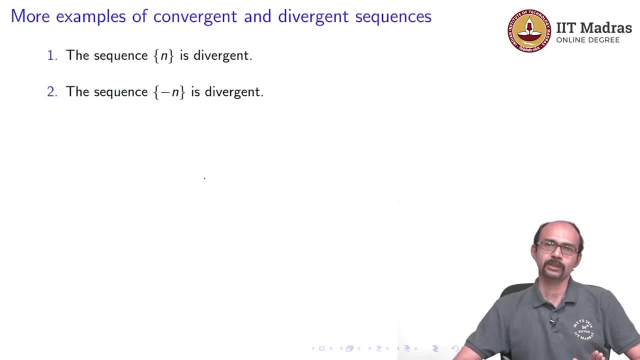 And if you take any real number, eventually the sequence will cross that real number. So if you take, let us say, minus 1000. Then if you look at the 1000 term, that is minus 1000.. If you take the next term, that is minus 1001, minus 1002, minus 1003, minus 1004, and you 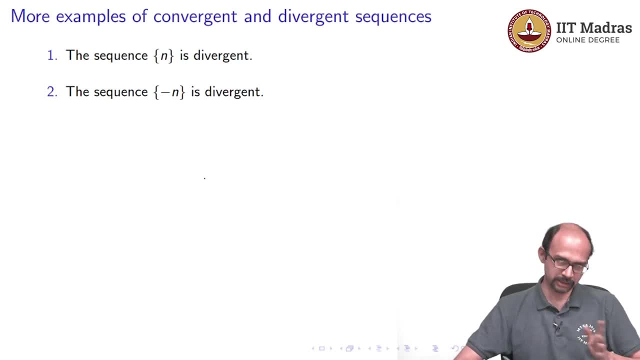 have gone beyond, You have gone smaller And it keeps becoming smaller. So it does not come close to this number, And that is true of any number. So it cannot converge to any real number, It cannot have limit any real number, Right? 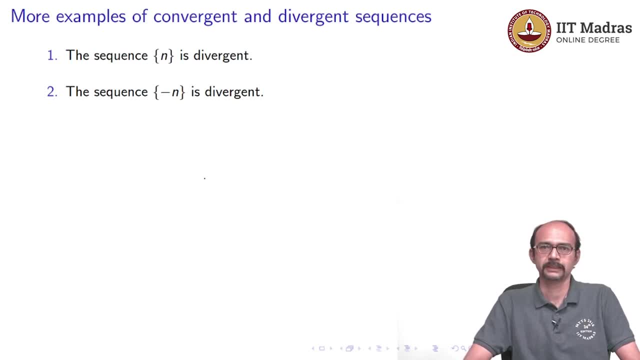 Now again, if you have heard of this concept of minus infinity, which is sort of on the other side of the real axis, it is what is called, what colloquially we say it is smaller than any number, any real number that we know. 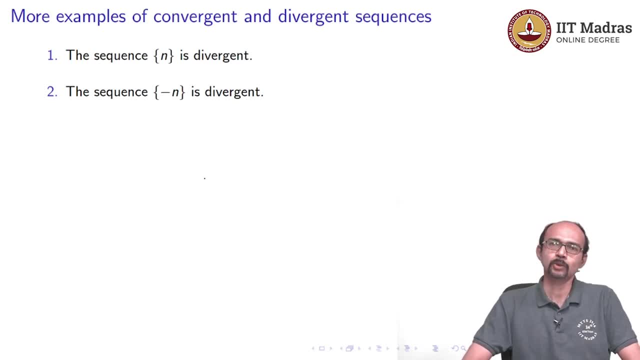 Then you can say that this sequence diverges to minus infinity or it converges to minus infinity. Both are equally valid and depend on the context. or you can just say the sequence minus n is divergent. Now I want to point out that these two sequences, n and minus n, are different from the other. 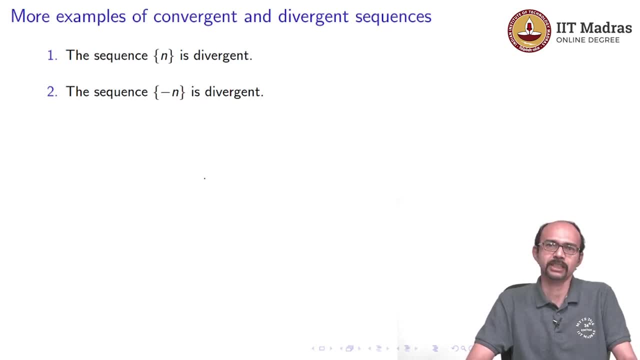 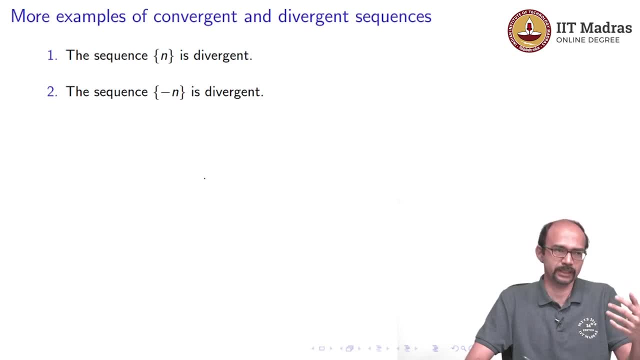 It has no concept of, it really does not converge in any sense, Whereas these sequences, they are really going off. Yes, So maybe they are going to something which is beyond our universe. where is, which means to say that our universe is a real line and it is going beyond that. 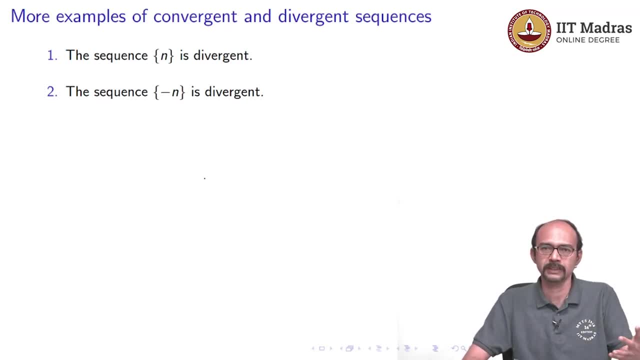 So there is a slight difference in these two types of divergence, but that is some pedantic point that we can ignore for this lecture course. Those who are interested in mathematics can think more about this. Let us look at some more sequences. So here is the first example of what is called a series, which I have made into a sequence. 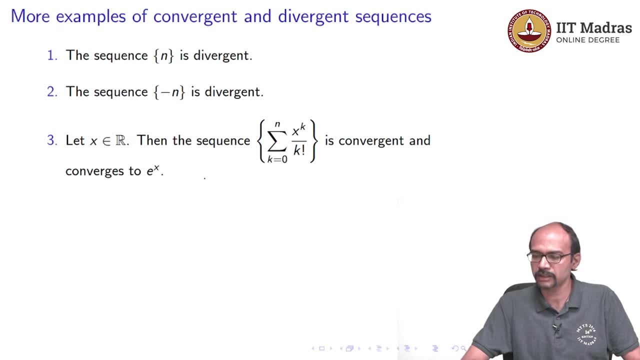 So you look at this sequence. What is this sequence? It is a sequence summation: x to the power k by k factorial. So the nth term of this sequence is this sum. So, for example, what is the second term? The second term is x to the power 0 by 0 factorial plus x to the power 1 by 1 factorial plus x. 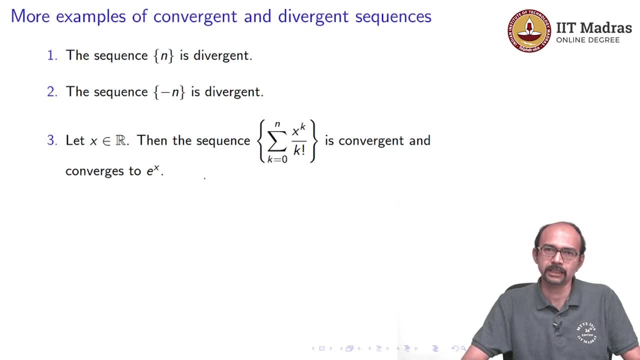 to the power 2 by 1 factorial. That is the second term. So if you have seen the exponential before, you can observe that if n tends to infinity- this is just summation- k is equal to 0 to infinity, x to the power k by k factorial. 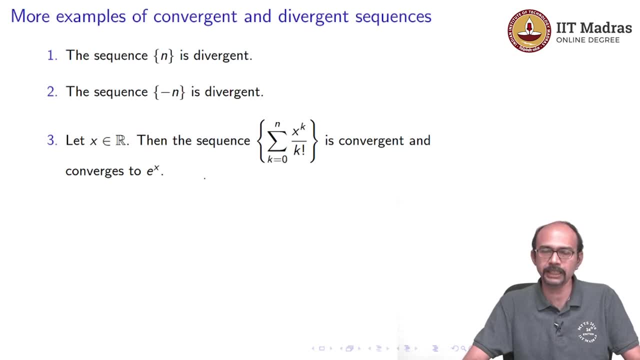 which is exactly what we call e to the power x. This is how we define e to the power x. So e to the power x is defined as: whatever this number is, Okay, Well, of course, you can ask: well, if I know what is e, then why not raise it to a? 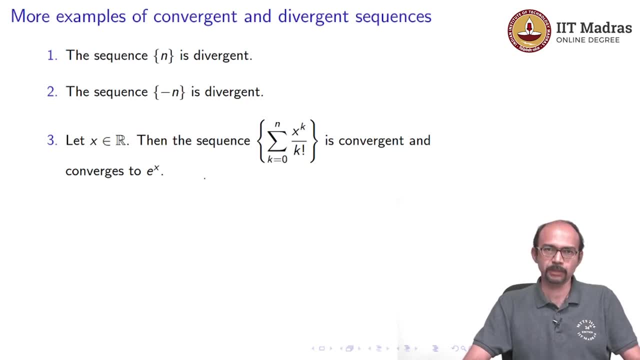 power? Certainly that is correct. But then what is e? And e is indeed defined in this way, by taking x to be 1.. So if you take summation 1 by k factorial, that is exactly the number e. That is how you define the number e. 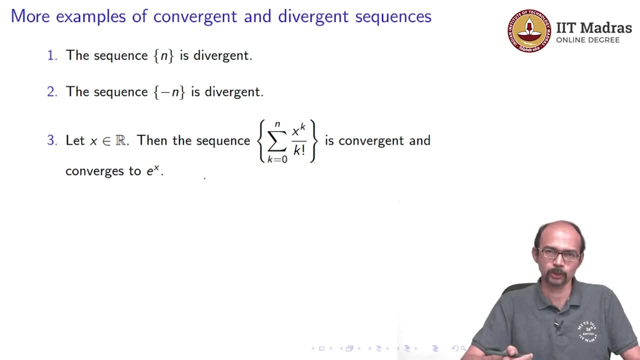 And then you work out what the value is, which is what Euler did, and so on. That is why it is one of the reasons it is named after him. Okay, Thank you. So keep in mind this is e to the power, x. that is what you need to remember. 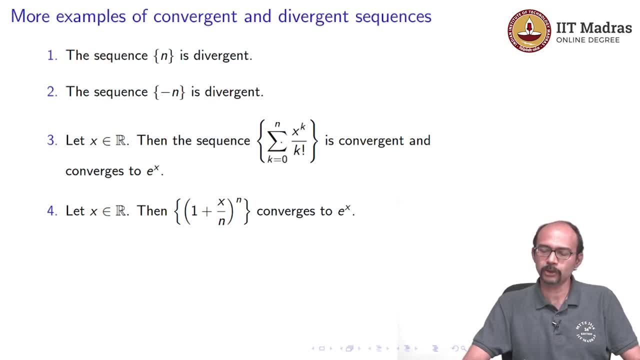 Similarly, if you take the numbers 1 plus x by n to the power n, then this converges to e to the power x. So the limit of this sequence is e to the power x. So what are the terms in this sequence? 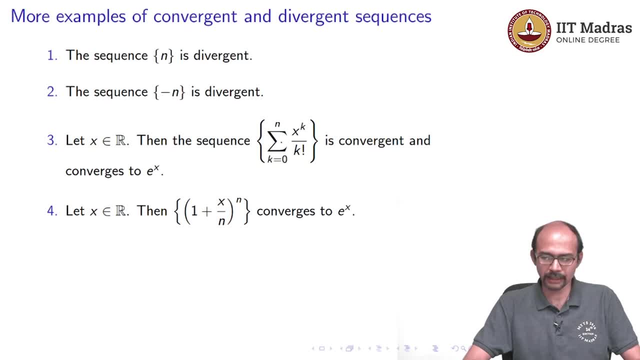 If you take x, if you take n to be 1, then this is 1 plus x to the power 1.. If you take n to be 2, then this is 1 plus x by 2 to the power 2, and so on. 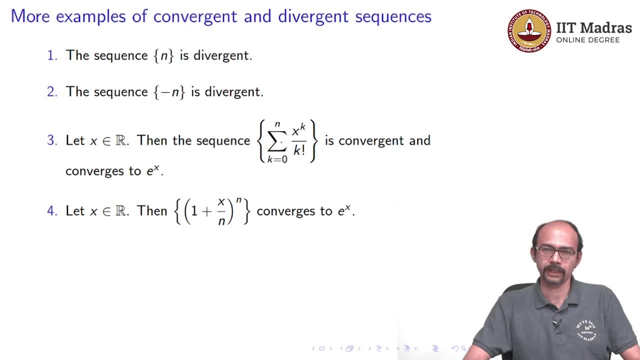 Okay, Okay, So this sequence converges to e to the power, x. Now this is you may. if you are seeing limits for the first time, I am sure this is appearing a little daunting. The point I am trying to make is: do not try to figure out why this limit is e to the power. 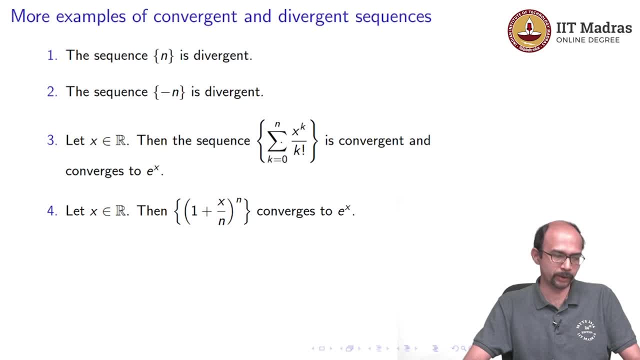 x. So you take these as a black boxes, that this is e to the power x. And then, similarly, here is something that you may see in statistics, which is why I have mentioned it. It comes about in some proofs in regarding this: 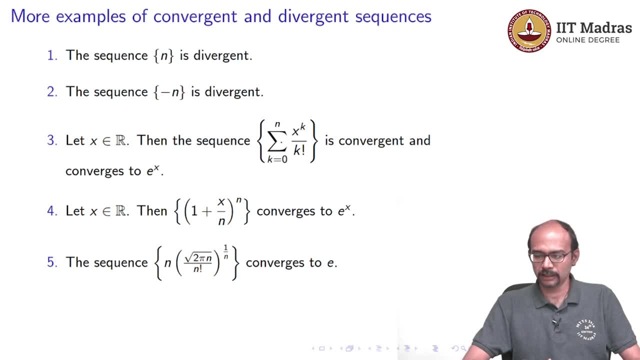 In regarding the normal distribution and so on, something called Sterling s formula. So from there, whatever that is, you can tell that the sequence n times root, 2, pi, n by n factorial whole to the power 1 by n very complicated looking sequence, converges to: 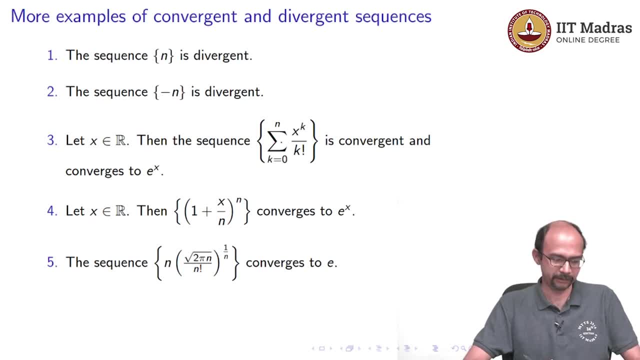 e something we know Again, black box, keep this in mind. And similarly, we have n by the nth root of n, Okay, Okay. So n by the nth root of n- factorial, again converges to e. So you can see that these notions of sequence are very useful and important because, whatever, 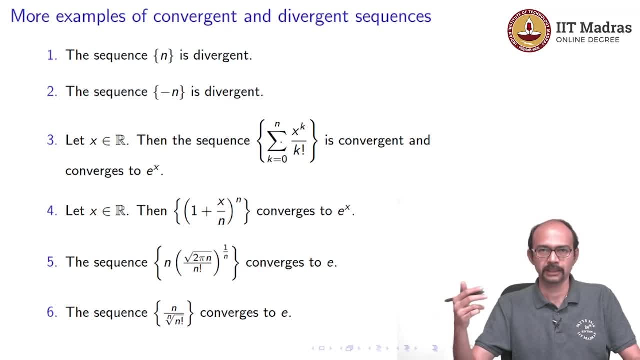 this thing, e is the exponential which we have seen, which is something which comes up in many, many, many places. somehow. it is very important in mathematics and statistics and science and technology, Okay, And at its very heart is this idea of sequences. 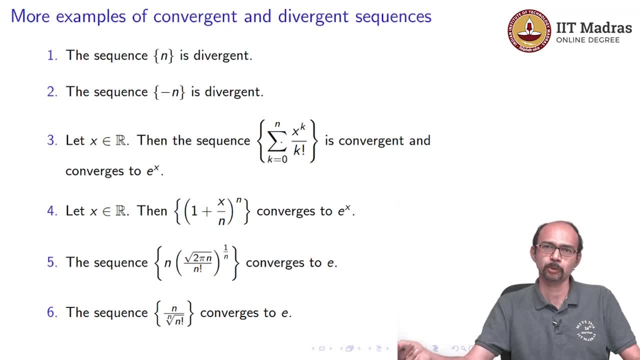 So you cannot really escape from sequences. So every time you are doing an exponential there is some sequence in the background. Only thing is we know how to deal with it And that is why we do not keep repeating it all the time. But I want you to understand that behind exponentials is this notion of sequences and series. 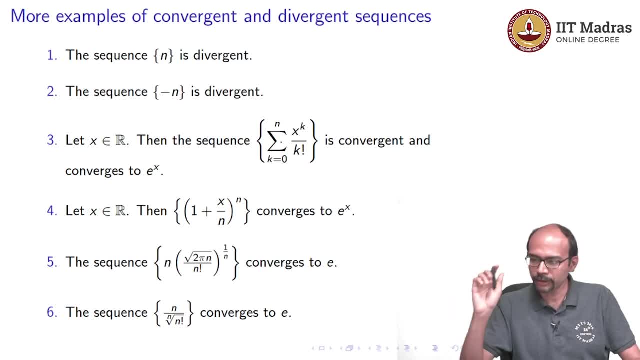 And you do not need to understand it very well. What you need to understand is: there are these sequences- Okay, There are these sequences for which the limit is the exponential function, or e, And that is what you need to keep in mind. Okay, 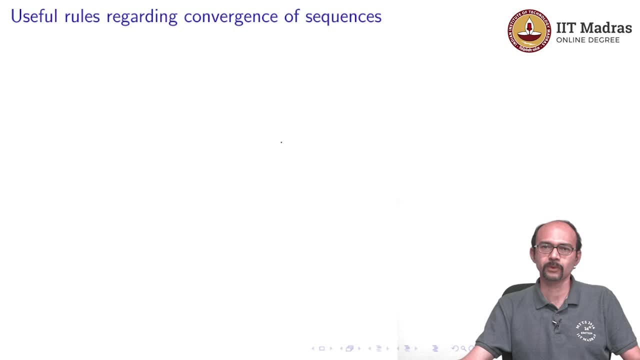 Fine, Let us write down some useful rules regarding convergence of sequences. This is what really helps: to know when a sequence converges So often, what will happen is: you will have a sequence and you want to know whether it converges or not, And well, you cannot keep evaluating. 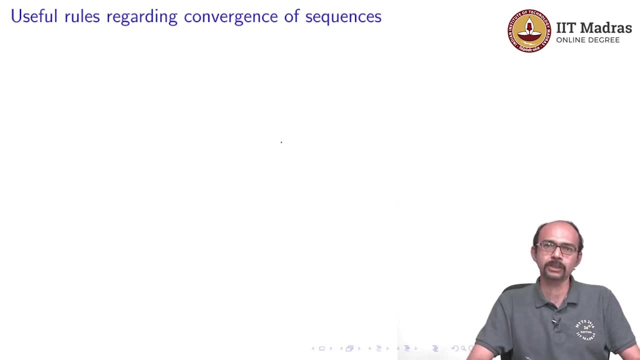 Right. What we did in our first few slides was we took the sequence and we took large n and we plotted it and we saw: how did that red dot move? Is it moving close to something? Is it not moving close to something? You cannot really do that. 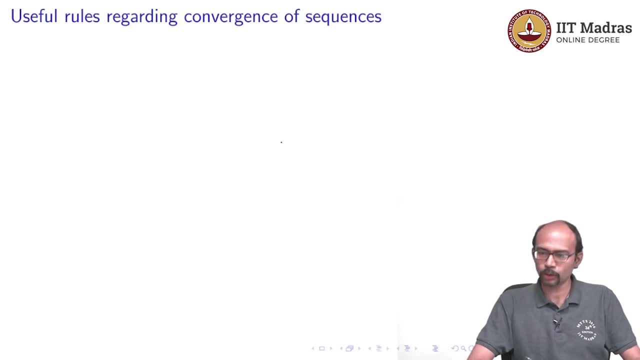 Even in the third example, which was 1 plus- sorry, 2 minus 1 by 1 plus log n whole to the power 1.1, you saw it moved so slowly that you really do not know it moves to 2.. 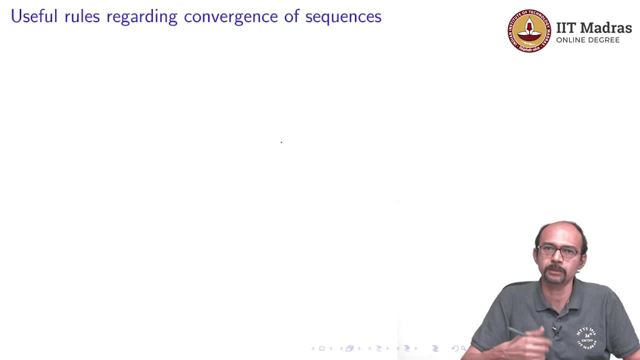 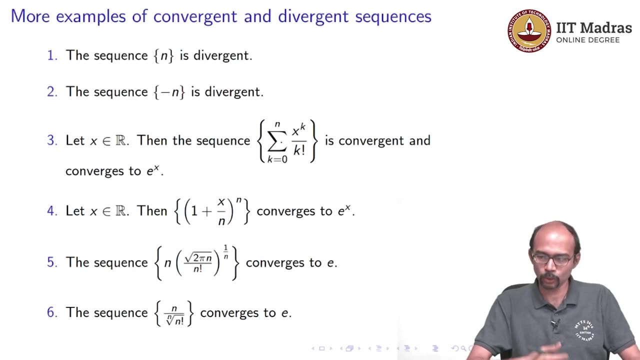 How do I know it moves, it converges to 2? So we should have some theoretical way of seeing that, And indeed that is what we will do. We will have some sequences for which we know what the limits are. Those were exactly the sequences we have described before. 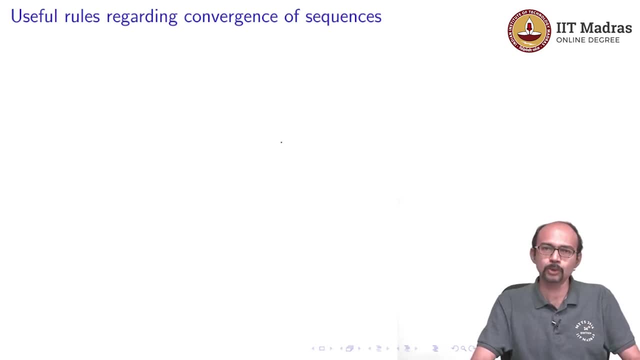 And then we will use those sequences to study other sequences and these rules and try to determine when they converge or diverge. So here is one, some such, here are some such rules. So if a n tends to a, then every subsequence of a n also converges to a. seems very logical. 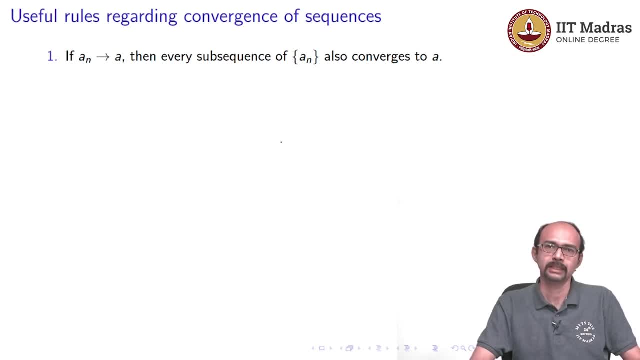 Okay, If a sequence is going to a, if you throw out a few terms and take the subsequence given, that will also converge to a. If a? n tends to a and b? n tends to a, then the sum converges to the sum. 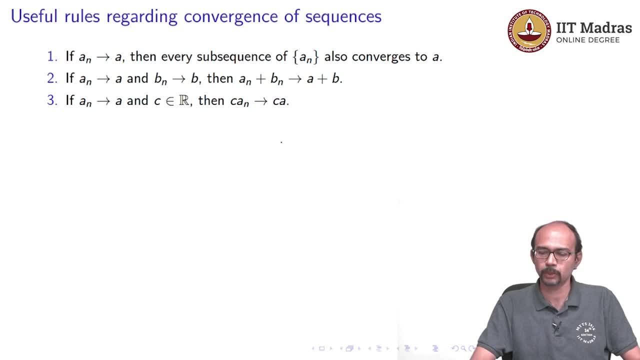 So a? n plus b? n tends to a plus b. Similarly, if you have a? n tends to a and you scalar multiply each of these numbers a? n by c, then c times a, n tends to c times a. a? n tends to a and b? n tends to b. then 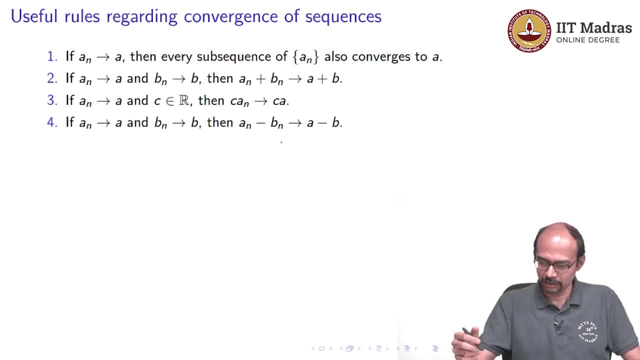 a n minus b? n tends to a minus b. You can in fact determine, You can derive this from the previous two, two and three: a? n tends to a, b? n tends to b. then the product, which means a n times b? n tends to a times b, a? n tends to a and. 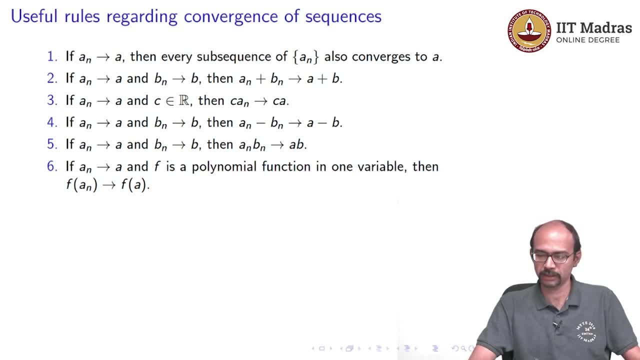 f is a polynomial function in one variable, very important. it is a polynomial function. Then f of a n tends to f of a. again, you can derive this from your previous, from 2,, 3,, 4 and 5.. 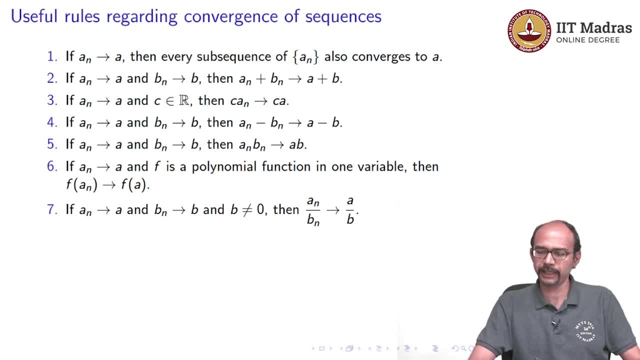 If a? n tends to a and b? n tends to b and b is not 0, very important- then a? n divided by b? n tends to a divided by b. So these are all rules. We have to prove these And indeed this is done in the first course on calculus, but we are not going to do it. 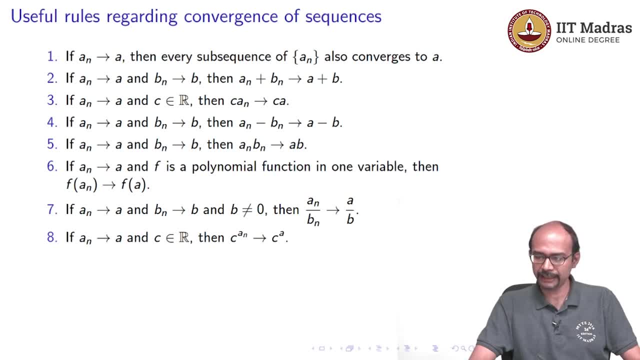 in this course: If a? n tends to a and c tends, c belongs to R, then c to the power a, n tends to c to the power a. Again something you can imagine, being true: if a? n tends to a and c is in R, such that 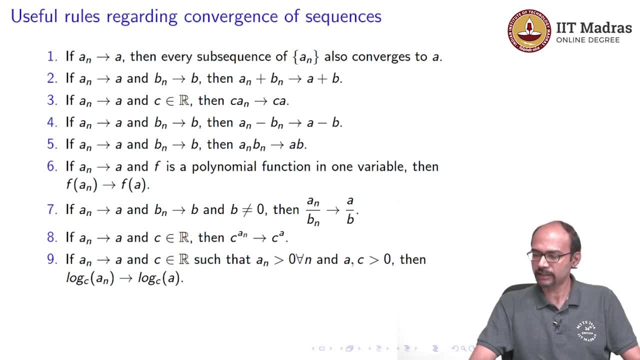 a? n is positive. So a? n is positive for all n and you have a n. c is greater than 0. Then log of a n to the base c tends to log of a to the base c And finally, this is a very useful and important principle called the sandwich principle. 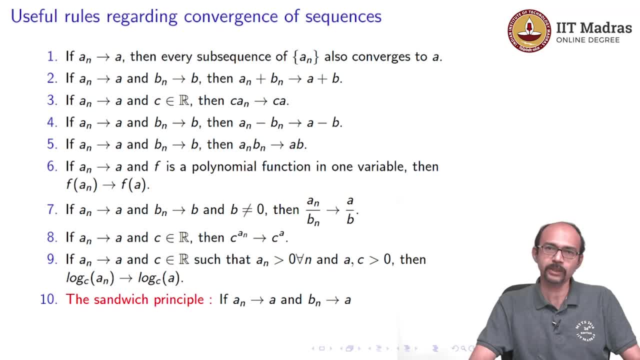 So if a? n tends to a and b? n tends to a, so you have two sequences tending to the same number, They have the same. these sequences have the same limit. So a is the limit for a? n and a is also the limit for b? n. 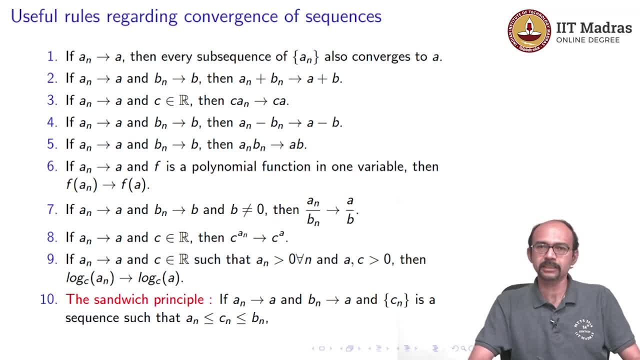 Now let us consider: and Cn is a sequence such that Cn is between An and Bn, So here is An and here is Bn and Cn is the middle. Then, as you can see, if An and Bn tend to something, Cn will also tend to that thing. 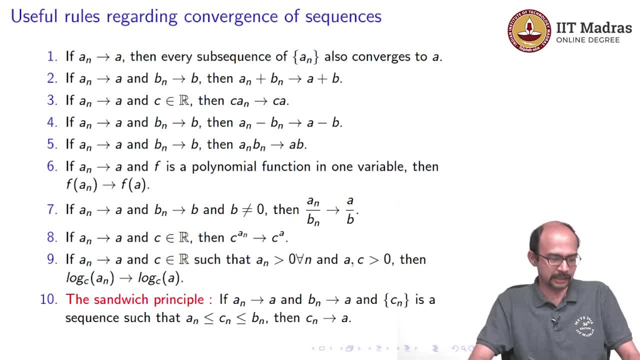 That is exactly why it is called the sandwich principle, So Cn is sandwiched between An and Bn, And if you use these 10 rules and some known results like the ones we described before, most of the sequences that you have to deal with are really can be dealt with using them. these 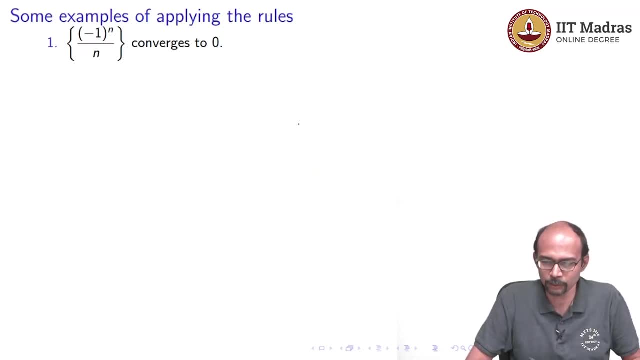 rules. So here is two examples that I am going to give you about applying these rules: Minus 1 to the power, n divided by n converges to 0.. And the other is some complicated looking expression like this: log of 1 by log of 1 plus n plus 5n squared by 1 plus n squared. 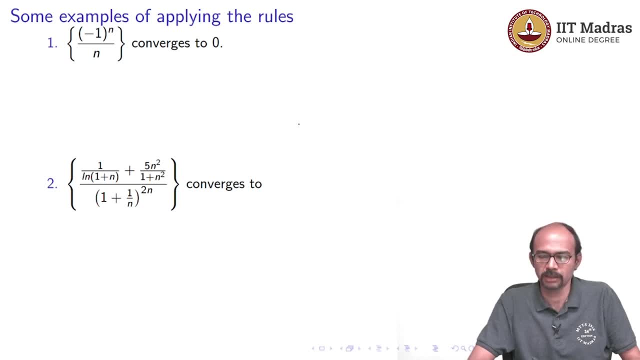 squared, divided by 1 plus 1 by n, to the power 2n, What does it converge to? So let us work out what these numbers are. Let us take the first one. So this is an alternating thing again. 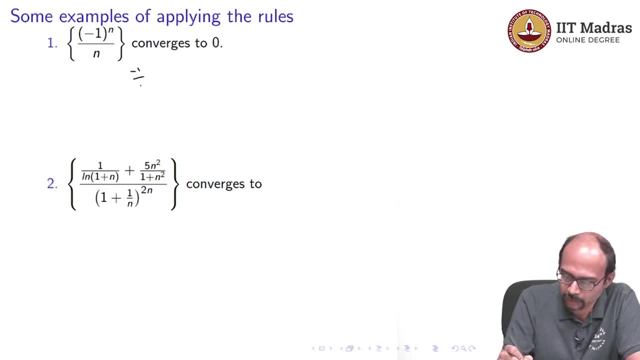 So the first few terms here are: minus 1 by 1, minus minus 1 by 2, minus 1 by 3.. So this minus minus 1 is just plus. so I will just write a 1 half. 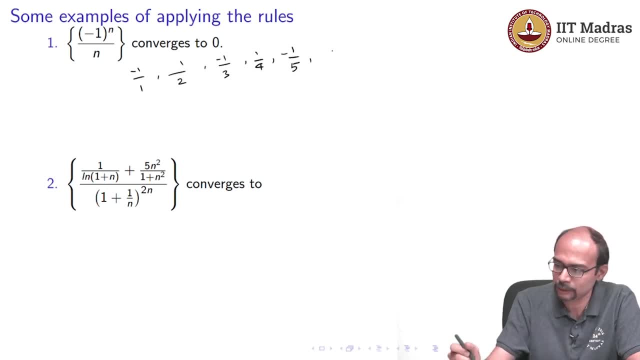 Then 1 fourth minus 1 fifth, and so on. So you can see, as the numbers increase, as n increases, these numbers actually come, although they oscillate about 0, but they come closer and closer to 0.. You can keep going. How do I prove this? Well, you can apply the sandwich. 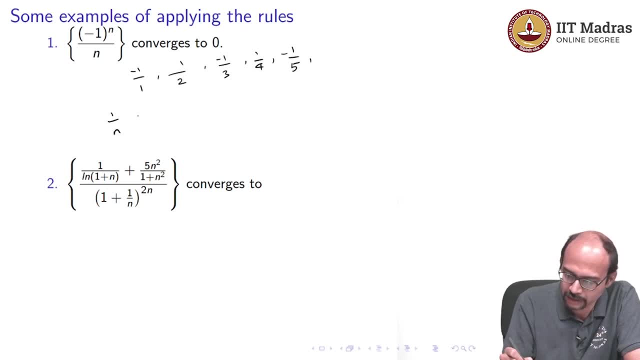 principle. First, let us look at 1 by n. We know that 1 by n tends to 0, that was something that we described before- Not given a proof, because I have never defined what is the limit- but this is something we know and we can intuitively feel. 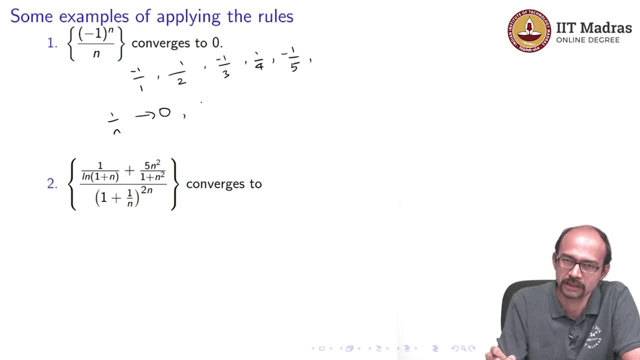 Well now, if you multiply the entire thing by some constant c, then it will go to c times the limit. So if I multiply this by minus 1, this goes to 0.. And now let us look at this sequence. So you can call this an, you can call this bn. both of them tend to 0. 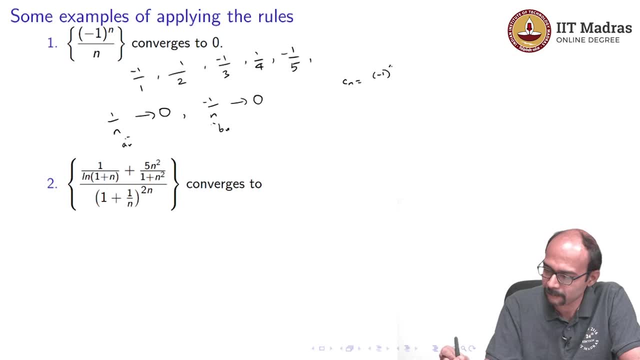 So you call the sequence that you have as cn And you can see that maybe you can call this, maybe I should call this an and I should call this bn, And you can see that cn is between an and bn. And now, if you apply the sandwich principle, this goes to 0,. this goes to 0,. 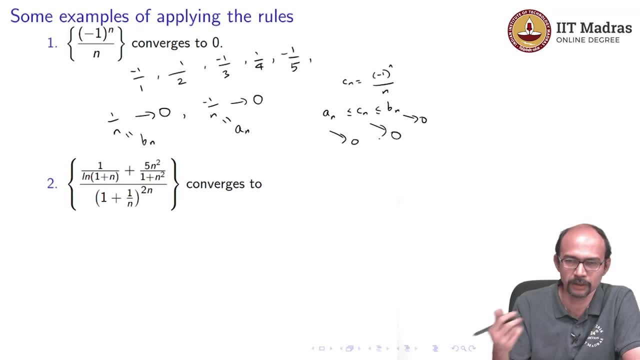 so this also goes to 0. That is how we prove this. I am giving. there are many ways of doing this, but I am giving you one way. How about the second one? So, for the second one, let us see. 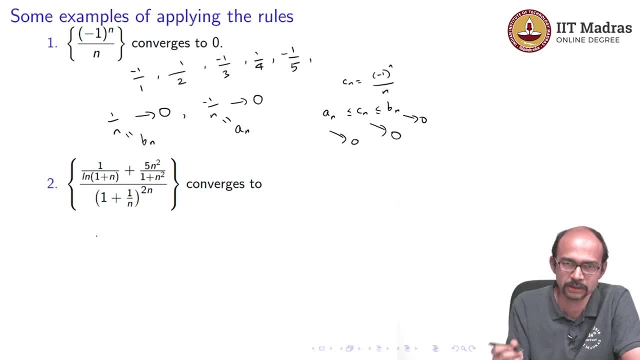 This is slightly harder, and I because it is not directly explained from the rules that I gave you, but I want to do it because I want to sort of explain what is going on. So let us look at log of 1 plus n. Well, n tends to infinity. what happens to log of? 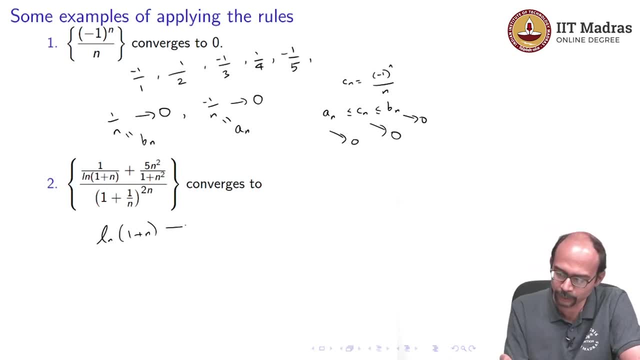 1 plus n. It moves very slowly, but it goes to infinity. This, so this sequence diverges to infinity. This tends to infinity, So diverges to infinity. Well, here is a fact. So, if that happens, 1 by this goes to 0.. So this part, so I know. 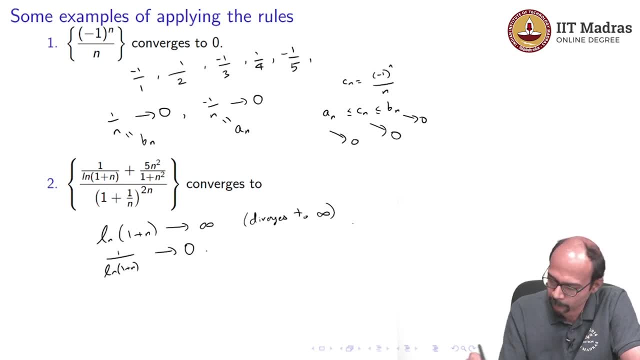 something about the first term and the numerator. what about 5n square by 1 plus n square? this is interesting. So here, if you can, you can look at numerator and denominator both separately. 1 plus 1 by n square goes to 1.. So that means here is a sequence. So I have 5 divided by 1, by n square, to infinity. so that is 1: n square. And then, finally, we are going to look at the second one, which is 1 plus n square by 2 plus n square. So 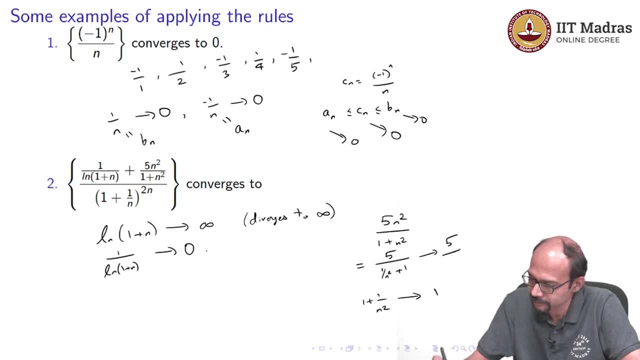 squared plus 1.. So this tends to 5 by 1, which is 5.. And now I have. so the numerator I have. I have kind of understood what happens. So if I call this an, if I call this bn, 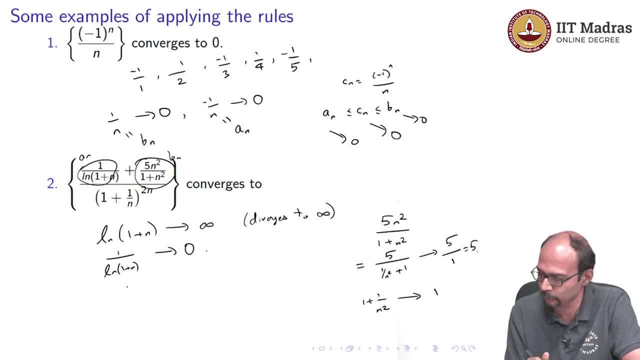 so I know what happens to an: an goes to 0,. I know what happens to bn: bn goes to 5.. So an plus bn goes to 0 plus 5, which is 5.. So the numerator goes to 5.. And let us look at. 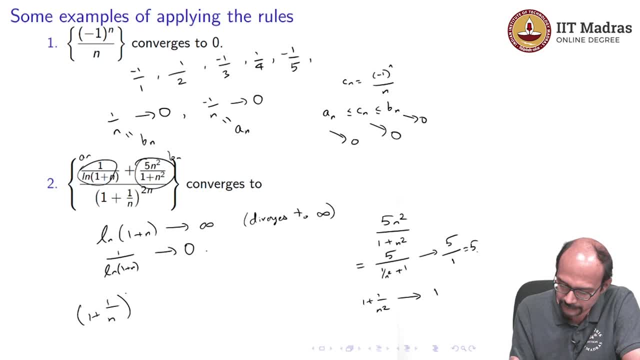 the denominator. So the denominator is 1 by 1 plus 1 by n by whole to the power 2, looks very complicated, But I can rewrite this as 1 plus 1 by n whole to the power n squared. And now I know what this term inside is. This term inside exactly goes to the number. 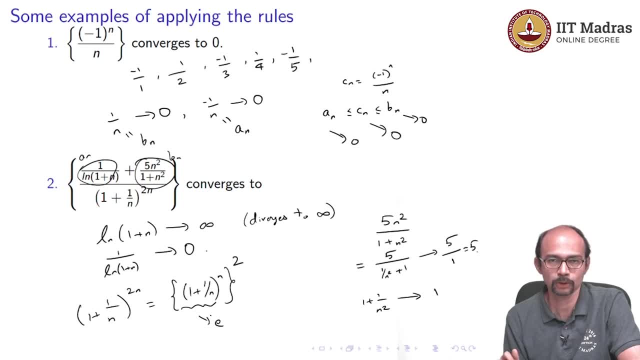 e. This was one of the things that we saw. So this goes to e squared. So in other words, this converges to 5 by e squared. Again, I am applying that if you take two sequences: an by bn. an tends to something, bn tends to something which is non-zero. 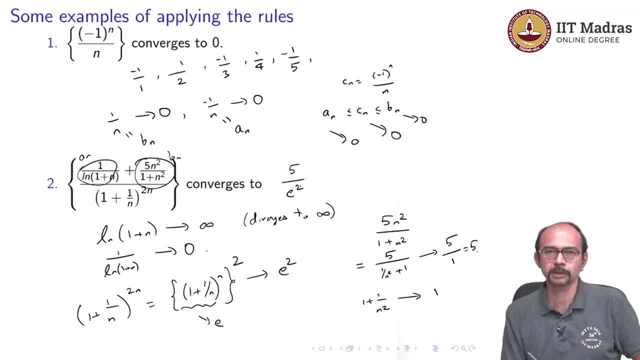 then an by bn tends to the ratio of the corresponding limits, So it goes to 5 by e squared. So this is how you are going to apply these rules and known examples in actual limits. So I hope this video was helpful. 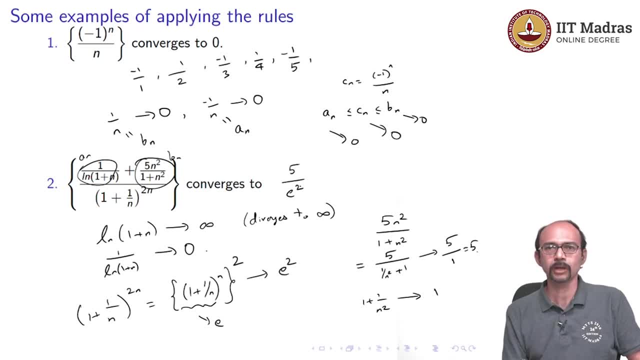 This video gives you an idea of how to, what is a limit and how to compute limits using these rules. So thank you.